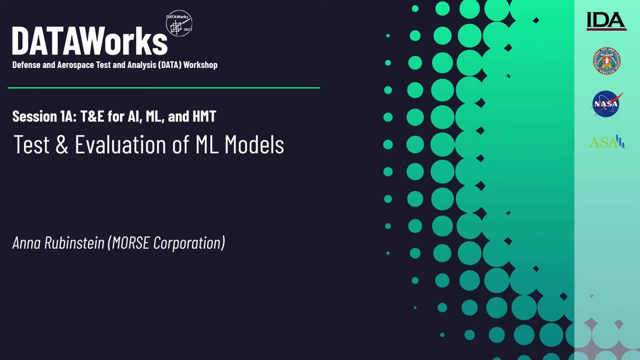 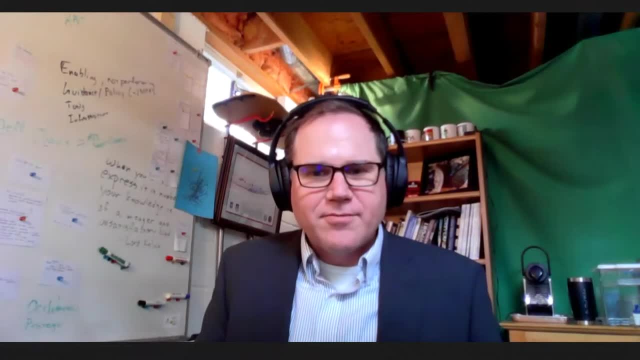 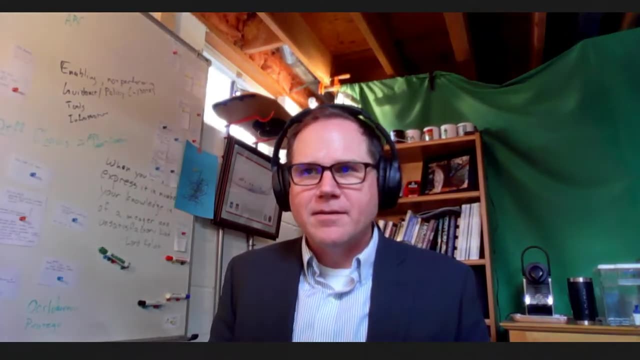 Next up we have Dr Anna Rubenstein. Dr Rubenstein is the current director of test and evaluation at Project MAVEN. You might have heard about Project MAVEN from one or more places, I believe. Defense News called it the flagship AI project in DOD yesterday. I've heard it called. 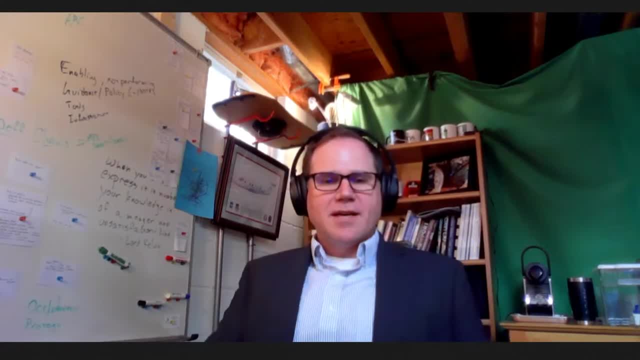 a number of other names also. Dr Rubenstein has a PhD in chemical engineering from Princeton. She previously worked as a science advisor at DARPA and a research staff member at IDA and has done work including development and testing algorithms for atmospheric modeling. 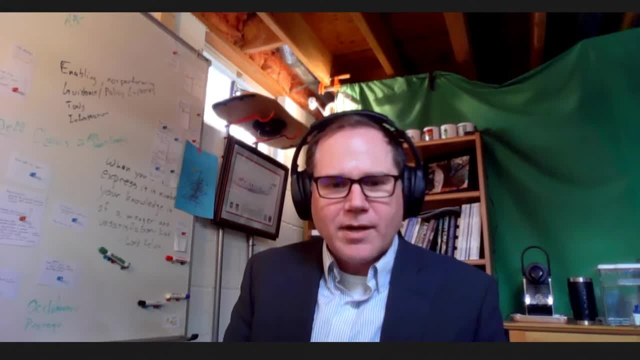 data fusion, social network mapping and nuclear weapons modeling- so a wide range of places. Today, Dr Rubenstein is talking to us about methods of measuring computer vision algorithms that support various different stakeholders. With that, Dr Rubenstein, are you ready to go? 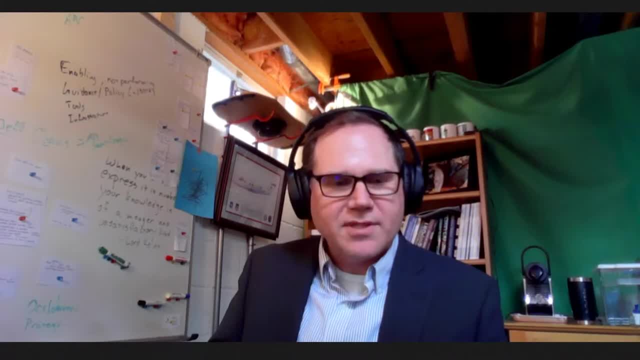 or do we need a little more space filled for slides to get set up? I think we're ready, but I don't know why the slides aren't showing Well while we wait for the slides to get up. I realize I didn't say anything about myself. 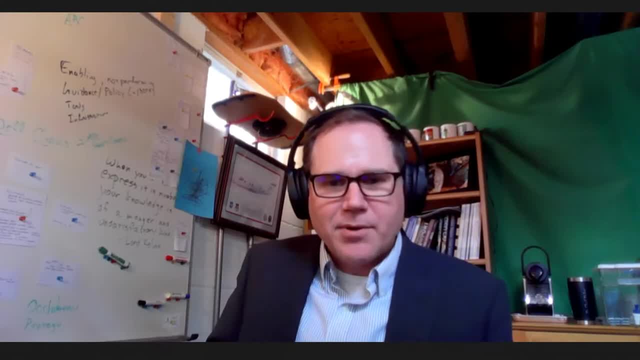 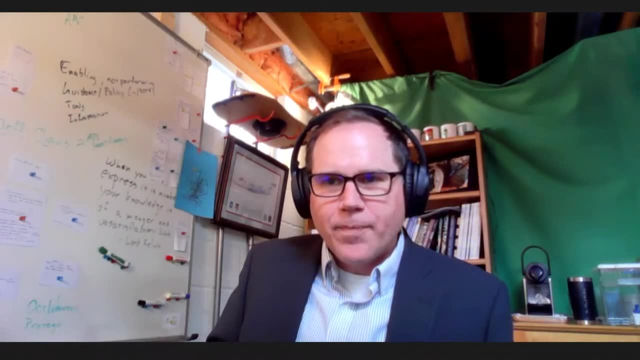 I just assumed everybody knew who I was, So I'm Chad Bieber. I'm currently the director of AI Assurance Operations at the Joint AI Center, working for Dr Jane Pinellas. I am sad that I couldn't be there in person, but COVID and other things stood in my way this year and hopefully 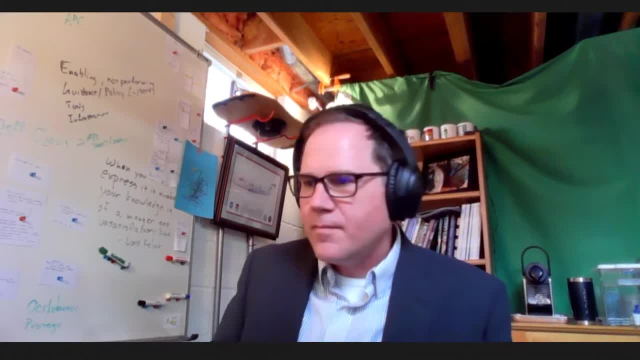 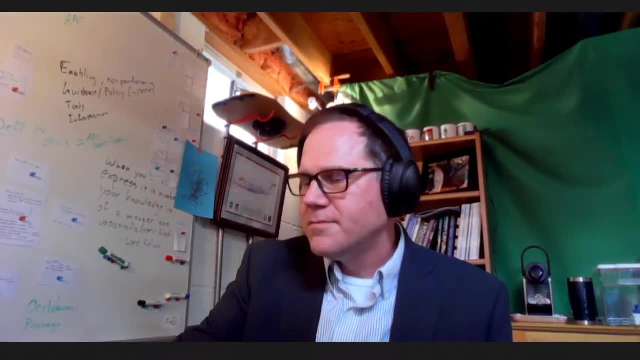 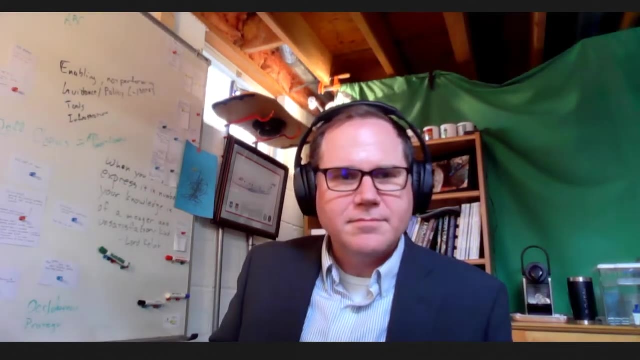 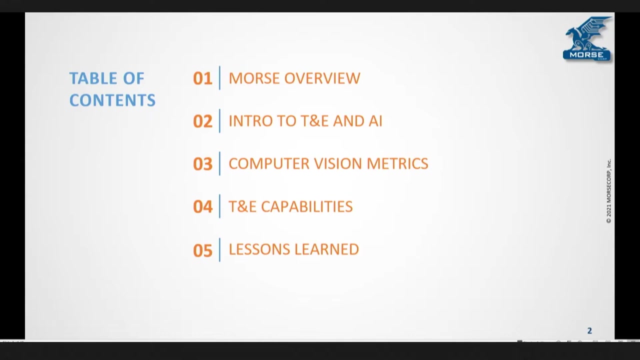 I'll get to meet in person next year at DataWorks. And where are your slides, Judy? Okay, Great, Okay. so thank you so much for that intro, Chad, So I'll jump right in. I want to take a couple of slides and just introduce the company that I work for, which is Morse. That stands for 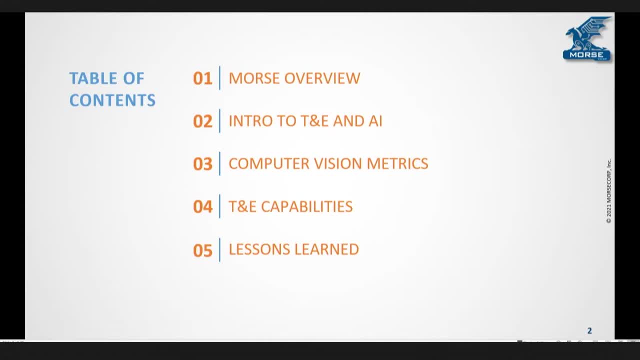 Mission-Oriented Rapid-Selective Networking solution engineering, And then I'm gonna give a little bit of an intro to T&E and AI. I'm not gonna spend a lot of time on this because Cornoli did such a great job in his presentation. 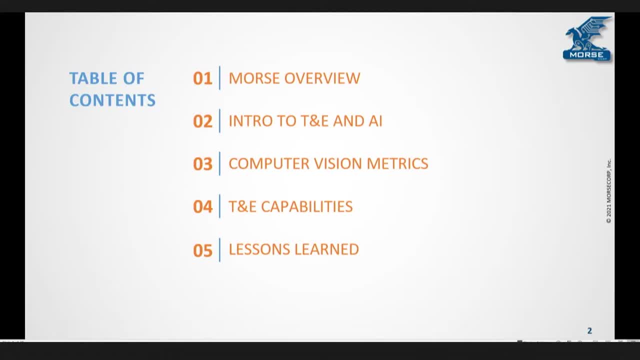 I can piggyback off a lot of that. The bulk of the talk is gonna be about computer vision metrics and why it's so complicated to pick the right ones for your use case, And then I wanna talk a little bit about T&E capabilities. 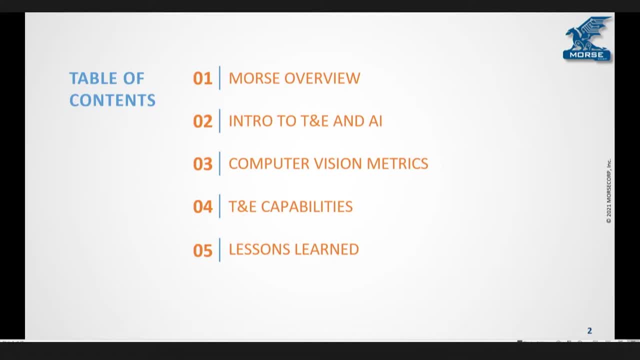 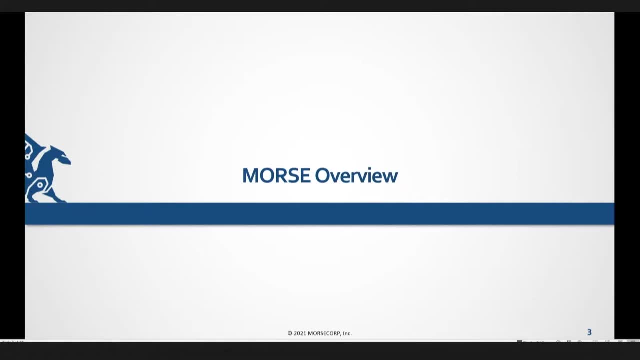 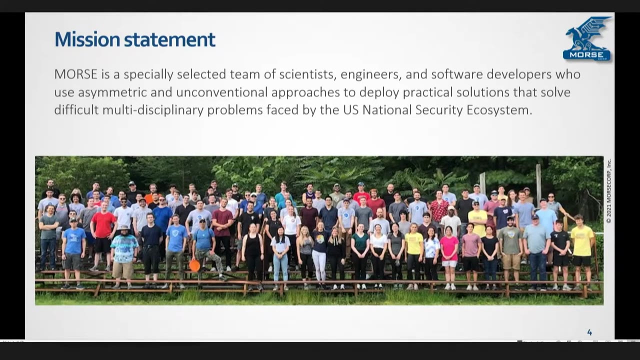 So actually, once you choose those metrics, how do you actually feel them and implement them and measure them effectively? And then, if we have time, we can talk about some lessons learned at the end. So, to introduce what Morse is, we are a small company of scientists, engineers. 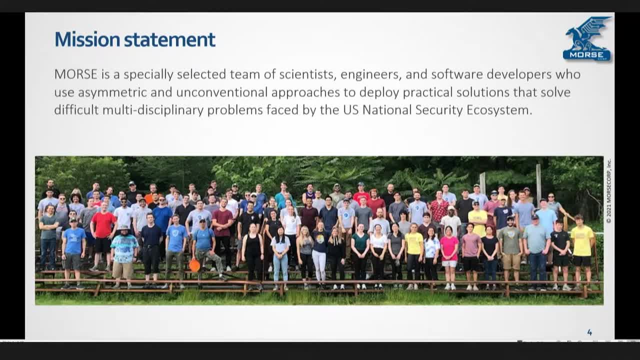 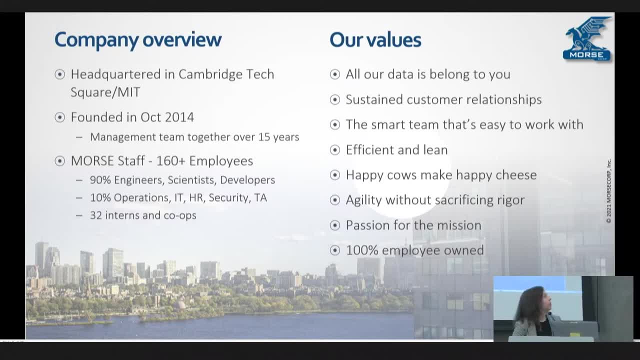 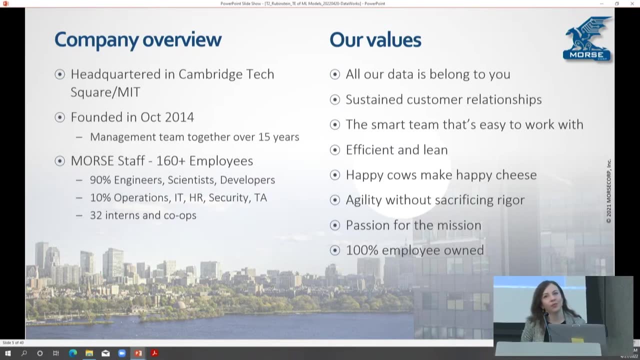 and software developers who work on problems for the national security ecosystem. We are located in Boston, I am not. I am here locally and always have been, And there are a number of values here that I wanna hold up, And I'm gonna use Morse as an example. 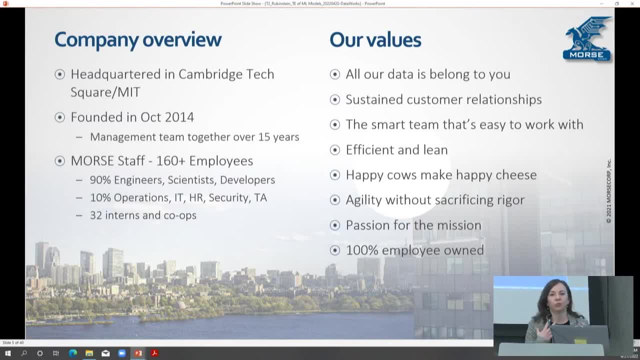 throughout this presentation, But not for the purposes of pitching Morse specifically, but I think there are a lot of values here and frameworks and lessons learned that are gonna be important and resonate with anyone who really cares about delivering T&E as a service, And I know that that's a lot of us here in this room. 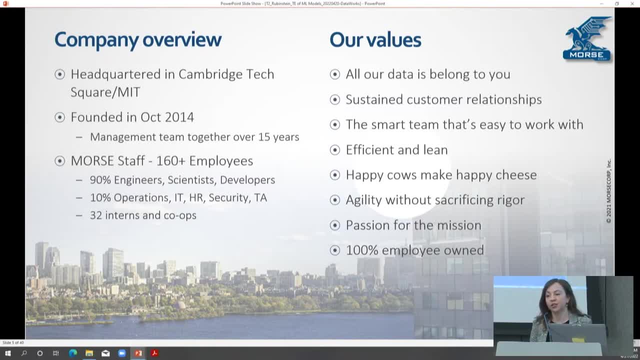 So all of the data and products that we develop belong to the government. We have no proprietary things that we hold dear. We share it with the government. We try to be smart, efficient, lean, happy, agile, rigorous and passionate and invested. 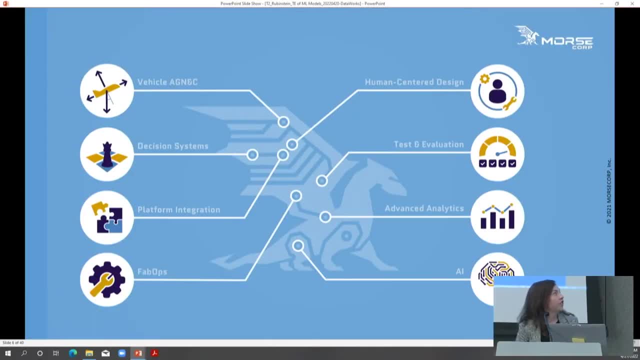 So that's why we're so interested in this mission. And then this slide just gives you a sense of the breadth of work that Morse works on. But we're primarily focused on this talk today on the T&E and AI portion, And here 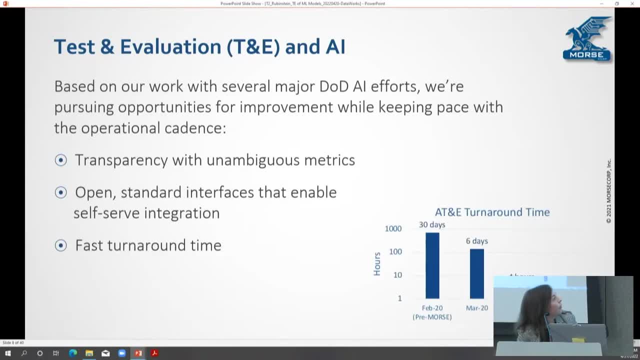 Okay, so introduction to T&E and AI. So the way we approach this at Morse is threefold. here We try to be transparent and have unambiguous metrics, provide to vendors and the government for decision-making. We have open standard interfaces that enable self-serve integration, so that kind of 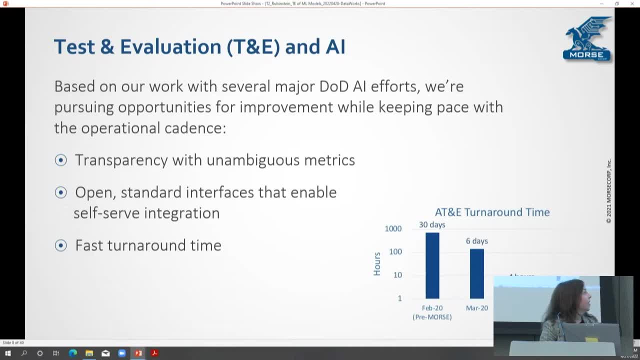 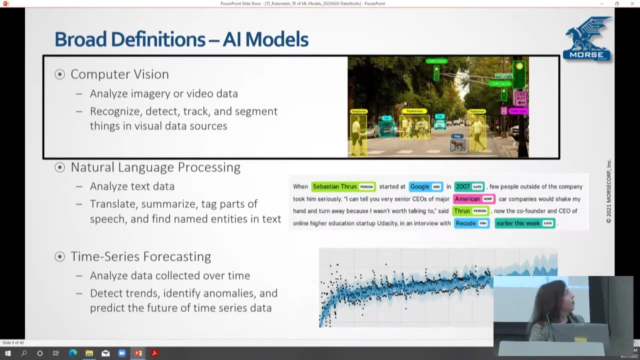 gets at that speed and scale pieces that are important to us and also that fast turnaround time. It's important to get that feedback as soon as possible so that vendors can react and work at making models that are more productive and useful to users. And then for this talk today. you know AI has a broad 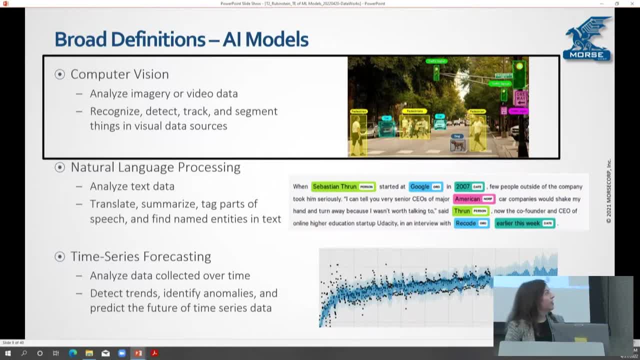 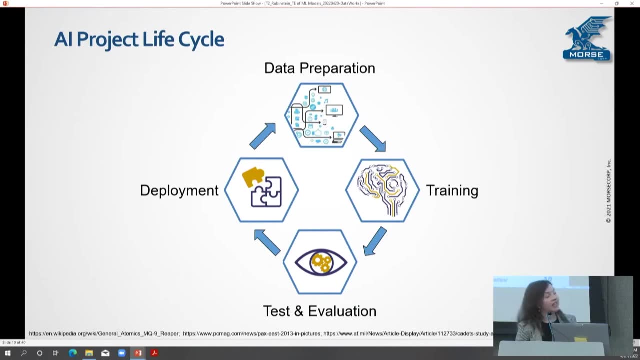 spectrum that it can cover. you know, natural language processing, time series forecasting, but here today I'm going to focus on computer vision and, even more specific than that, I'm going to be looking at object detection for full motion video as an example. And then, you know, within the AI project lifecycle, we 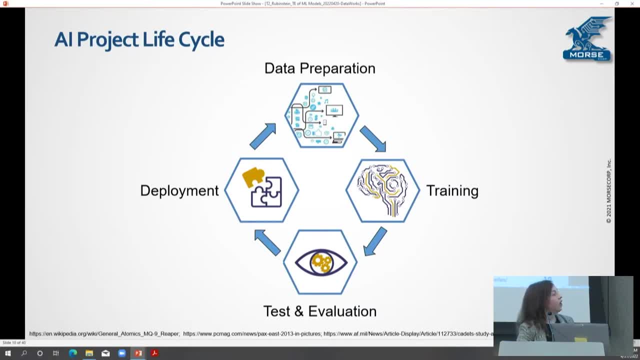 can see where T&E fits. you know it can often be used as a gatekeeper of figuring out which models are best for deployment, but then it needs to feed back into that loop. you know, taking, taking those lessons learned, taking that data back and really 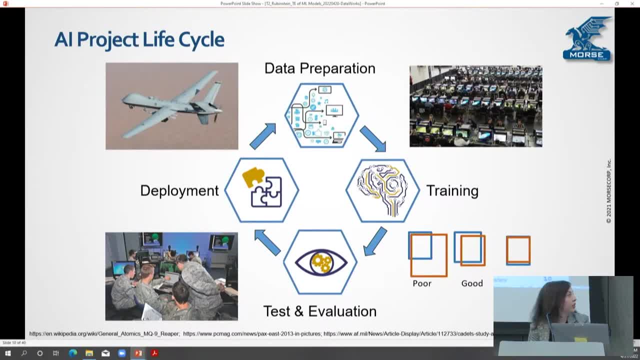 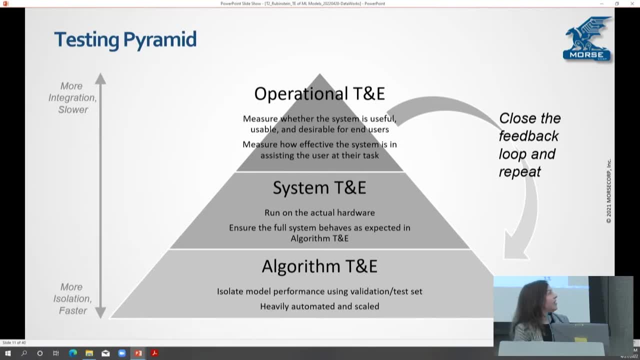 harnessing that to leverage the full capabilities that are available to your, to your AI model. And then here is showing the, the testing pyramid. Colonel Woolley presented this in a different format and actually broke his up into into four pieces. I do it in three and so we have you know algorithm T&E at the. 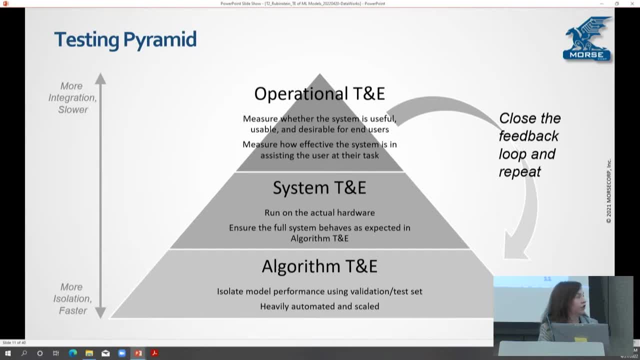 bottom, where that's your testing your models in your sandbox with your curated- you know- T&E data sets. It can be a heavily automated and scalable process When you have system T&E where you plug your models into the actual system, the hardware, the networks that it's going to. 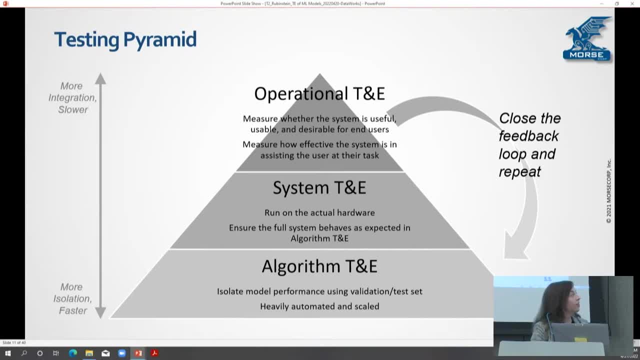 be running on making sure that you know you've actually implemented everything correctly and that it's still behaving the same way that you predicted in algorithm T&E, And then operational T&E, making sure that the system is usable, useful and desirable for the end-users. You know, is it making them faster? Are 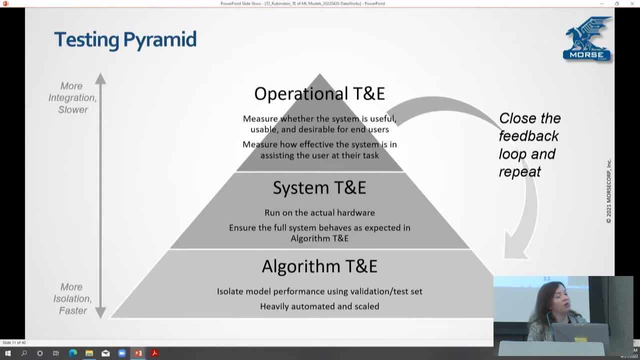 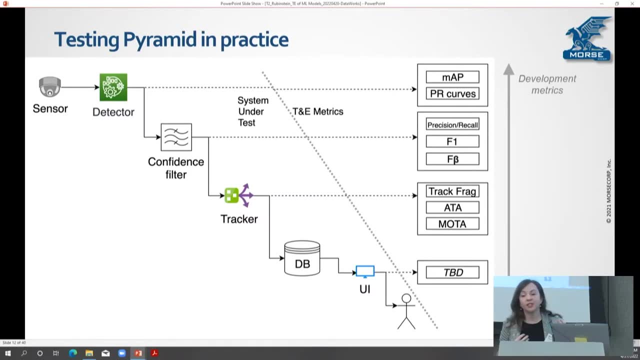 they finding more targets? Are they finding better targets? And then how do the humans and the systems actually interact together? And so, for the purposes of this talk, I'm going to dive a lot deeper into algorithm, T&E and the kinds of choices that we've had to make there to really 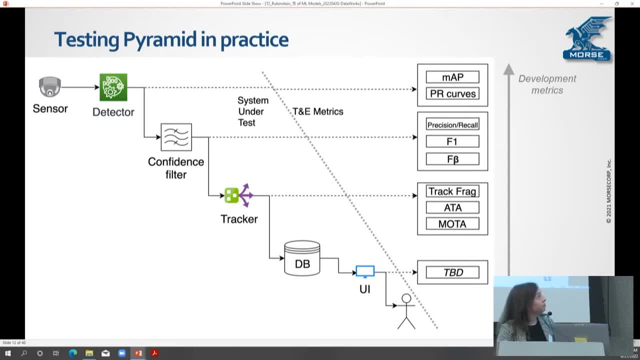 facilitate model development for the DoD, And so this shows you a picture of blowing out that testing pyramid and sort of peeking back under the hood of everything that goes into an algorithm, And you'll see that the right metrics choices vary depending on what you're looking at. which layer of capability? 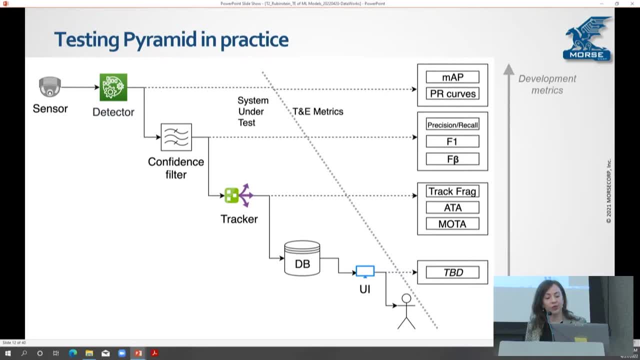 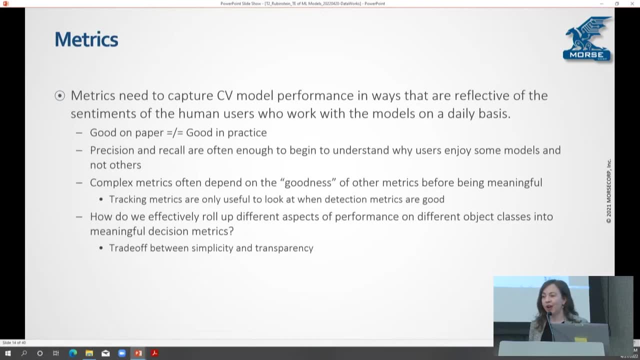 you're trying to test for, And so that is what I'm really going to dig into in this section. So computer vision metrics. So I might be preaching to the choir here, but I think this is surprisingly complicated. You know, it seems like it ought to be easy There. 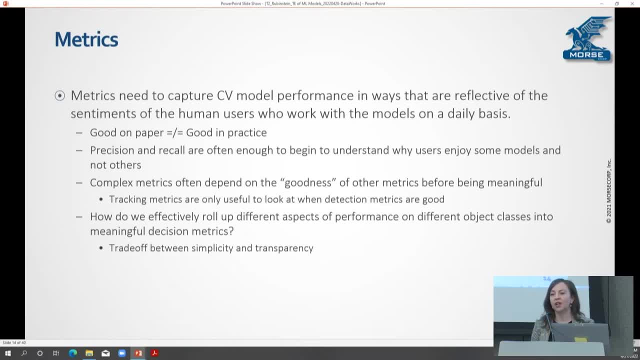 ought to be an objective, right answer, Like: what is the best model? Why can't you tell me? Why can't you tell me which one is the most accurate and why doesn't that you know? check all your boxes of what you're looking for. But it's really 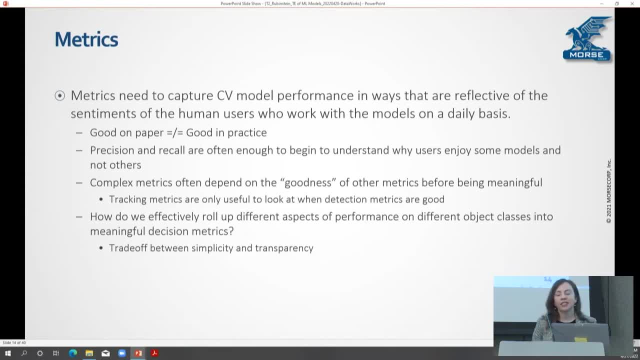 not that simple. And then you know, specifically for object detection models, accuracy isn't even defined. You know there is no concept of a true negative. So how do you even approach what best could mean? Sometimes you have to back into it using a few different metrics, And so you know what we've found is. 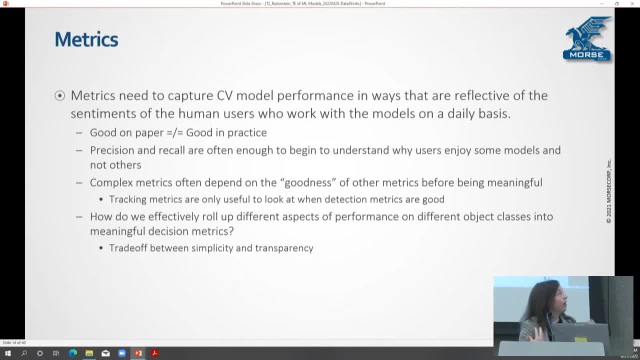 things that sound good on paper, you know, and that you know like great academics can come up with, like this is how you have to do it. A lot of times it just does not work in practice And you just discover that by trying it out and 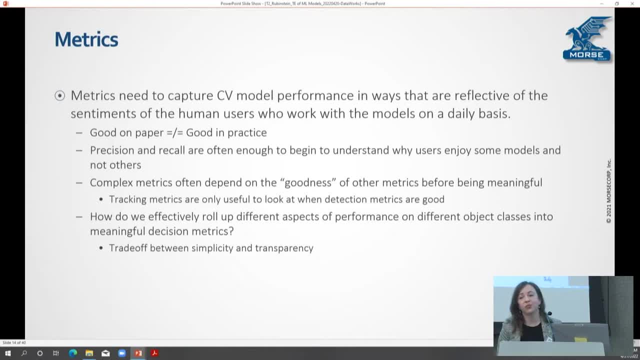 failing and, you know, trying again. So precision and recall are often really good jumping off points and they can start to give you an introductory understanding of why users might enjoy working with a particular model, but they they're not the whole story. 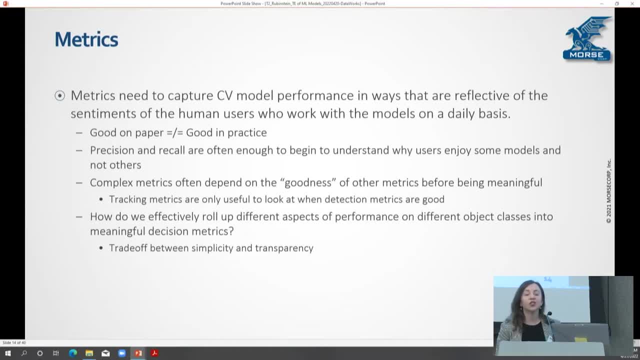 They're not the complete picture And sometimes you can't even get to those more complex metrics until you've already sort of established some basic level of goodness, you know, at a simpler level. So, for example, if you want to do tracking in a video, you 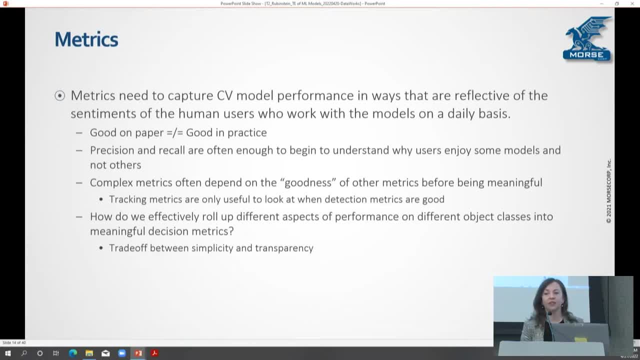 can't even, you can't even touch that conversation until you've gotten just basic, you know, within a frame, detection, correct, And then getting active. how do you answer that question? of which one is the best model? Sometimes you wanna roll up a number of different. 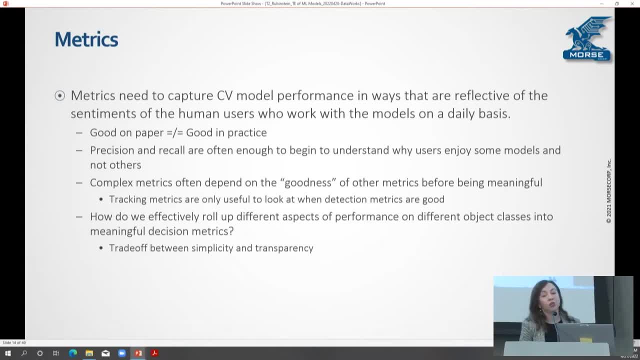 performance aspects into a single value that you compute. That's easy, that's simple to understand, you can point to it. But how do you really effectively do that, especially when you're looking at considering a number of different object classes And you get a real trade-off there between 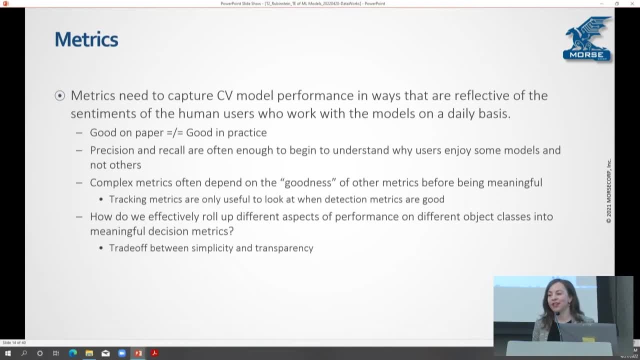 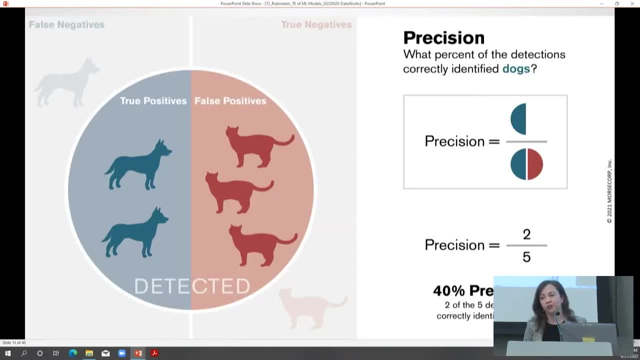 the simplicity of having a single number and then the transparency of understanding how that number devolves into a number of different aspects. So I'll start with defining precision and recall, because those are the two sort of building blocks of a lot of the metrics that we use in computer vision. 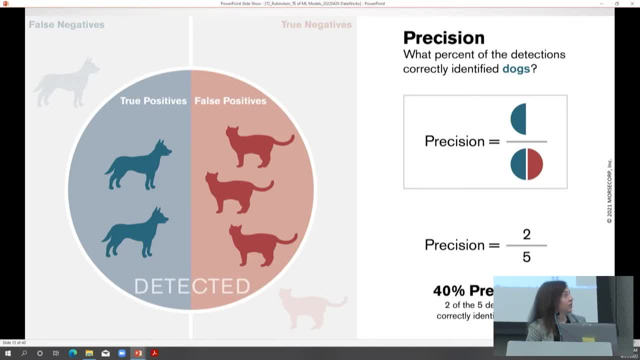 So precision tells you a lot about the quality of your detections. So in this example it's looking at what percent of the detections are correctly identified as dogs. So you see here two out of five, so two of the five detections are correctly identified. 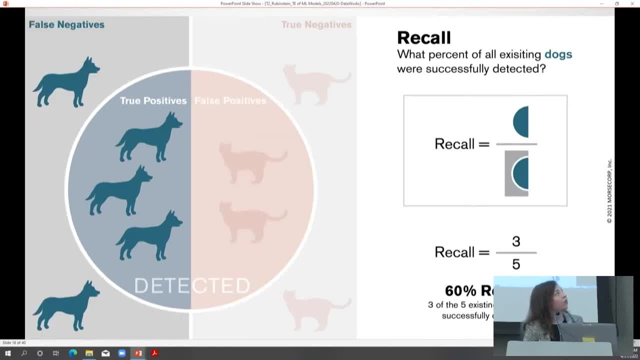 In this slide we're looking at recall. So that tells you more about the object class that you're particularly looking at. So here, what percent of all of the existing dogs were successfully detected? So here you can see that three out of the five. 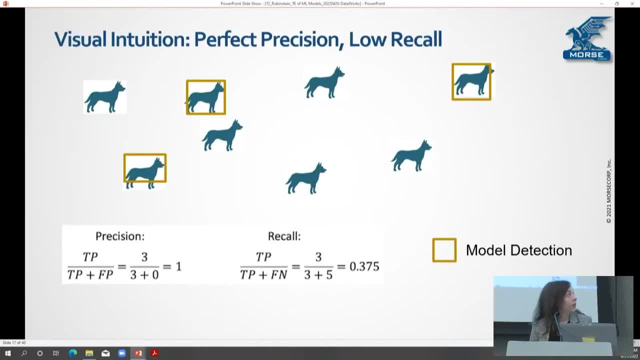 were picked up, so that's 60% recall. Okay, so that all makes sense, But what does that really mean? What does that look like when you start combining these features of a model together? So this example shows perfect precision and low recall. 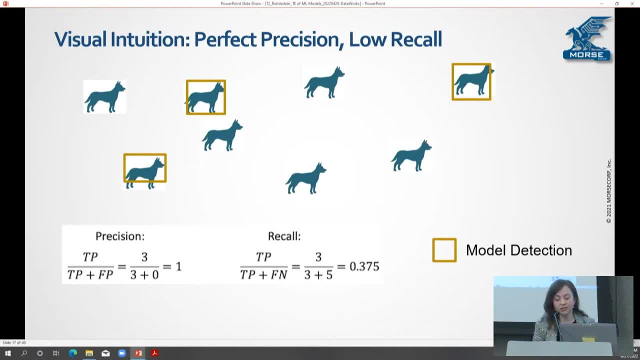 So you can see that everything it told you was a dog was in fact a dog. However, it missed most of the dogs up there. Is that sufficient model performance for you? I don't know. it depends on your use case, right. 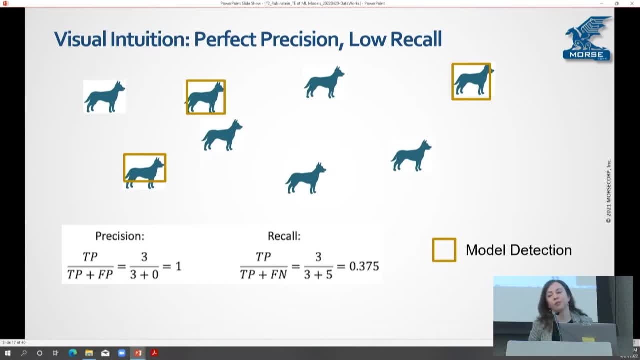 Like, if you only want to get that tip and cue from a model when it's absolutely sure it's correct, then this might work for you. However, if you absolutely have to be notified anytime there's the remotest chance that a dog is there, 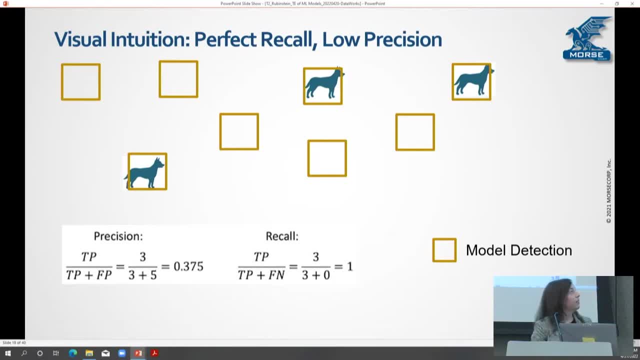 this probably isn't gonna cut it for you, So here's the opposite example. So this is perfect recall, low precision. So here it picks up every single dog on the screen. However, it's also flagging a lot of false positives for you. 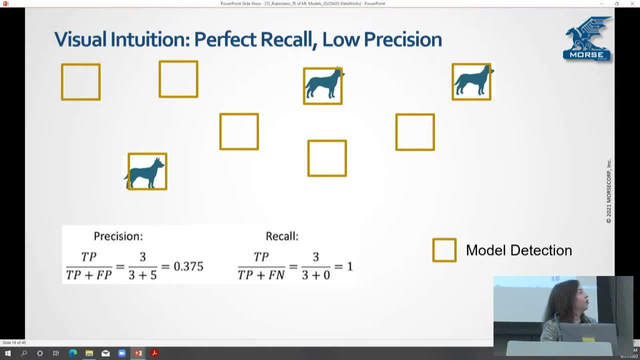 Is this acceptable for you? Maybe, maybe not. So it just really depends on what that use case is. which can make it complicated when you're trying to develop models for a general use case, because then you have to start making trade-offs. 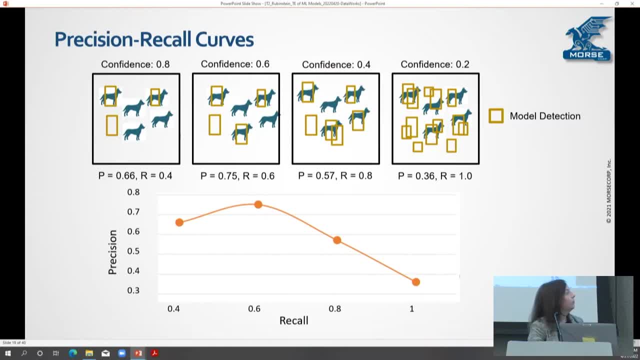 How do you balance these two? So one way you can understand that trade-off between precision and recall is with a PR curve, because the unseen third dimension here is the model confidence. So you can set different confidence thresholds and that will let you map out this full curve. 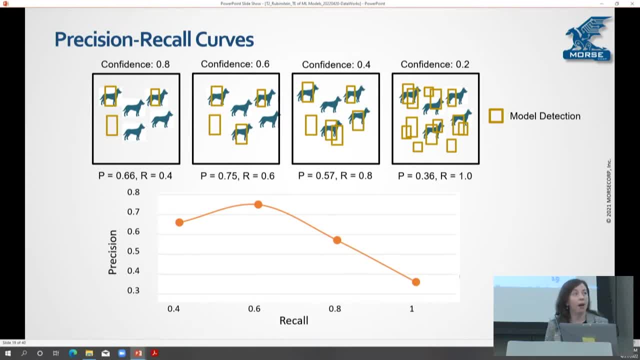 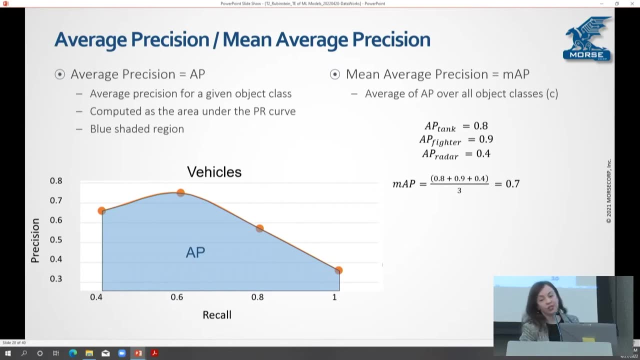 And that shows you the full range of capability of your model And that can be useful to model vendors understanding how they are performing in general. And then this is a really common metric that's often used for computer vision- is average precision, which measures that full shape under the curve. 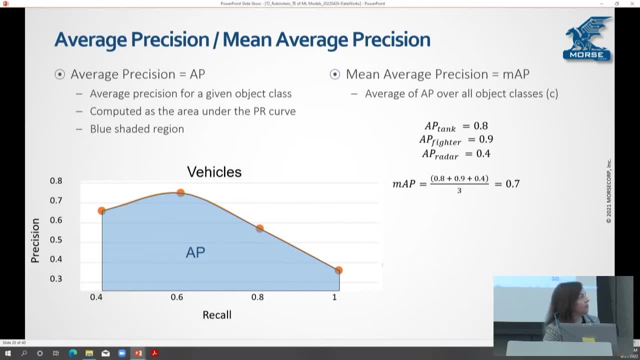 Mean average precision would be averaging over all the different object classes, your model output. So this is all well and good, but in a lot of cases the user never experiences that full breadth of potential model performance because the model operates at a single fixed operating point. 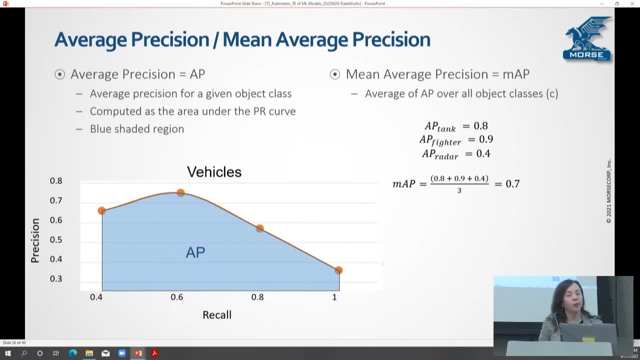 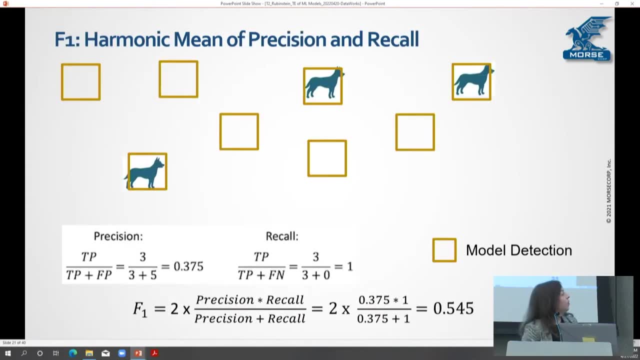 And so if you really wanna reflect and optimize around that point, the full curve doesn't matter, because the user's never gonna see that. So one way of getting at that operating point a little bit more directly is with an F-beta score. So here we're showing where the beta value would be one. 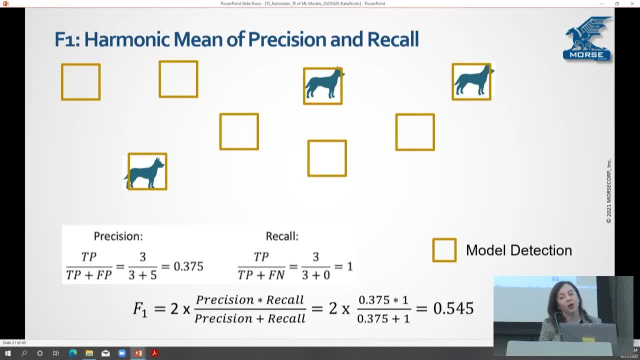 So this would be a harmonic mean of precision and recall, where precision and recall are equally balanced. So this could be a metric for a real general use case where precision and recall are equally important to you. So you can see, you know this behavior here. 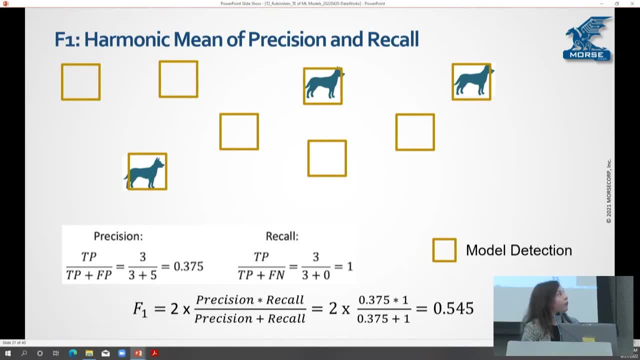 is giving you a value of about 0.5, 0.55.. And you know, and visually that could make sense to you right like it's getting about half of the things you care about a score of about 0.5.. 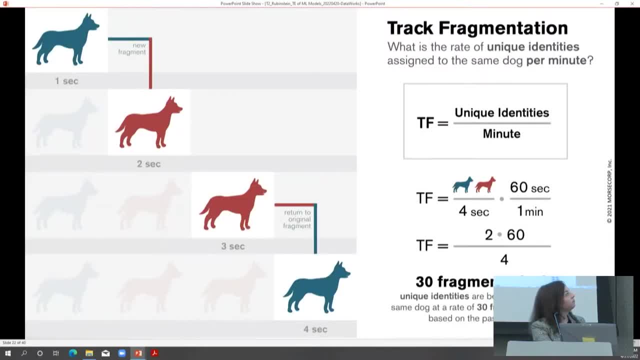 You know that resonates, that's easy to understand, It's intuitive, So but maybe that's not enough. If you're doing you know, if you're running an algorithm over a whole video, maybe you don't care, just 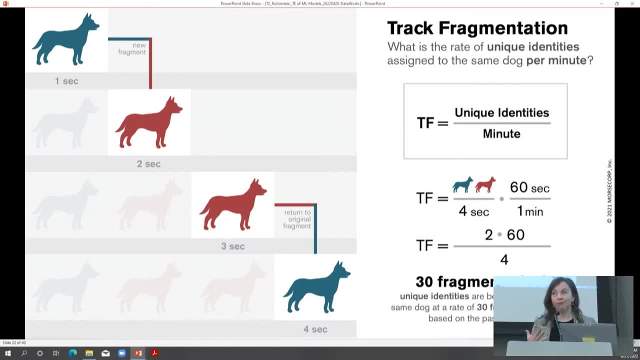 about that frame to frame importance. You know, academically that might make sense, but when you're actually watching the video, what if those detections are flashing in and out and now you're watching and out and distracting you and you're like man? I wish that algorithm could. 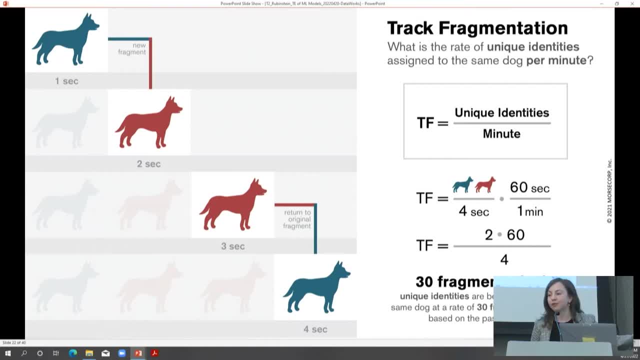 just hold on to something, hold on to the identification frame to frame and have that persistent identification so it's not flashing in my face. so this happened on one of the programs we work on, and so we started using this additional metric called track fragmentation, and so the the reason of starting to surface this. 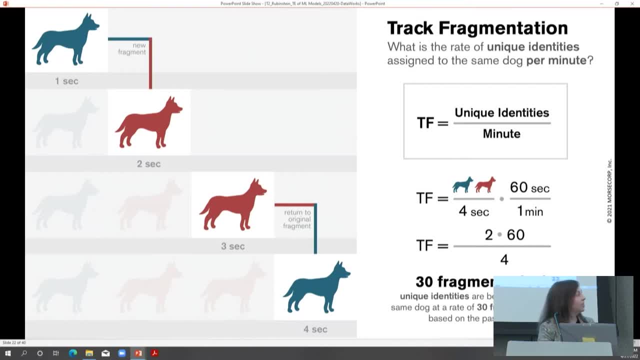 was to tamp down on that flashing, that ID switching that was so distracting to people. so this measures the number of unique identities assigned per minute. and so you can see in this example here, this would be 30 fragments per minute. per minute, so that would be a lot of switching. so so now you know we've. 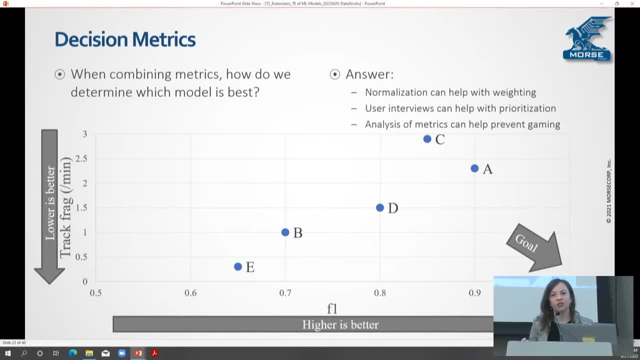 talked about a detection metric and a tracking metric. again, how do we start to roll these up into decision metrics when we're trying to decide what is the best model? and there are a lot of traders that are using this method, and they're using this method and they're. 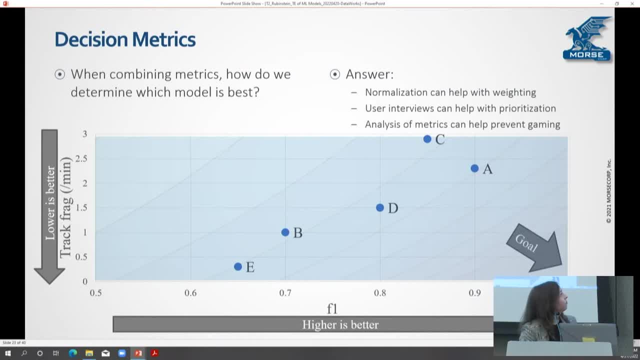 schedulers and they're farming and they're using this method and they're sampling their data and they're buying collected data expeditions, because now they're going right back into the field, while the important thing, we need to learn more from people and we need to teach people how they should dealing with 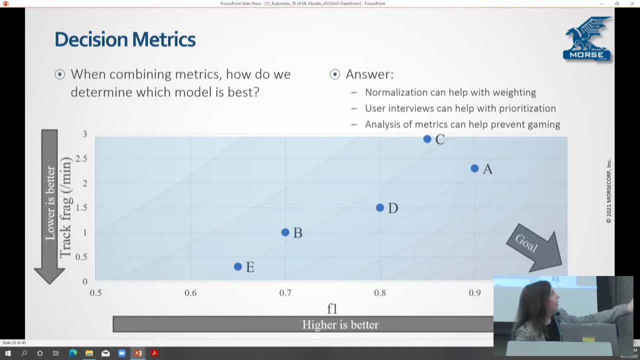 this. so, for example, go to bank year've Gary Stere Meiners major, huge one of his F-beta, So you can come up with strategies for normalizing even unbounded things. You have to pick a dampening factor and that can be somewhat arbitrary. Sometimes we don't like making these decisions, but we have. 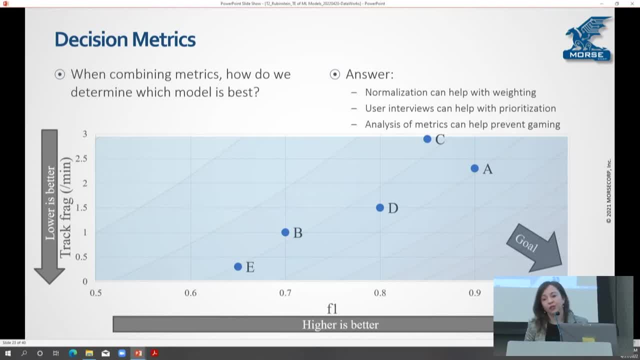 to, And then also user interviews can help you with prioritization, And so that's something that you and a lab can't decide. You have to take that to the users and get their feel on it, But they might be able to give you better insight on what that trade-off is to. 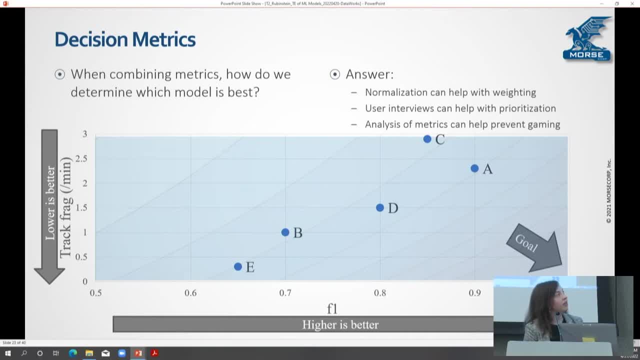 them between an F-beta and track frag, for example. And then, whatever solution you do decide on, you should do some robust analysis on it to make sure that there aren't gaping holes somewhere that you haven't considered. You don't want your metrics to be susceptible to gaming, where the 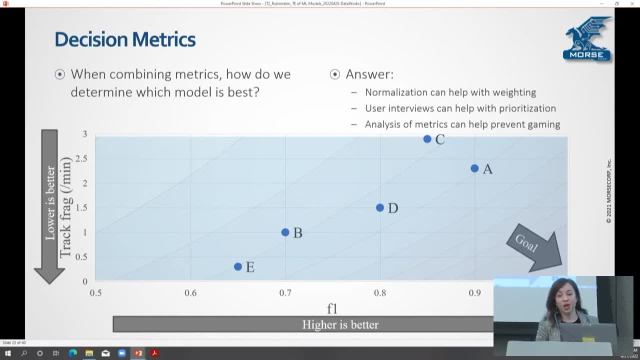 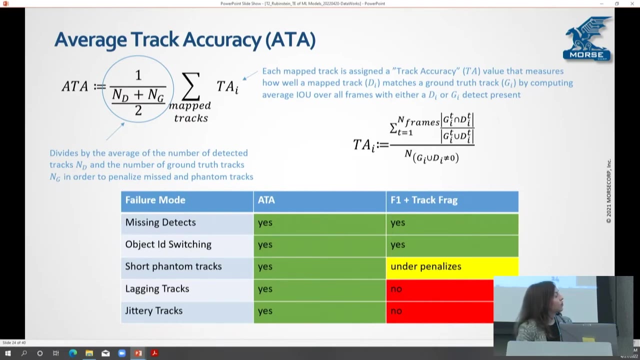 vendors could be meeting the mark in terms of the number that you asked them to optimize on, But by doing that they could be introducing a whole bunch of other behaviors that are really going to be detrimental to a user. So, once you've accepted the level of complexity up to this point where we're 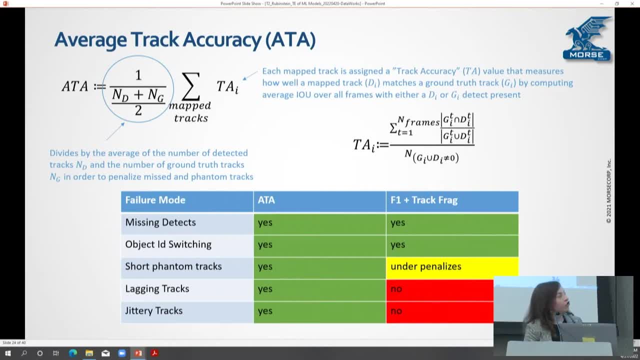 trying to find a better way of doing detection and tracking. an additional, more complex, more comprehensive metric that we looked at is average track accuracy, So I don't have a pretty slide here with dogs to explain this one. It's getting more complicated, But it measures how well a map track matches a 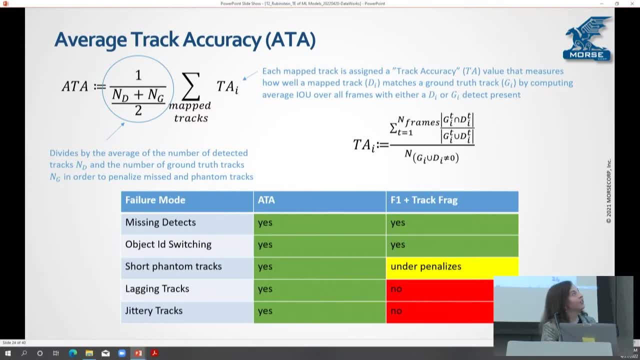 ground truth track by considering the average IOU over all frames And it scales by the number of detected tracks and the number of ground truth tracks as a way of penalizing missed and phantom tracks. So you can see a head-to-head comparison here of these two different types of 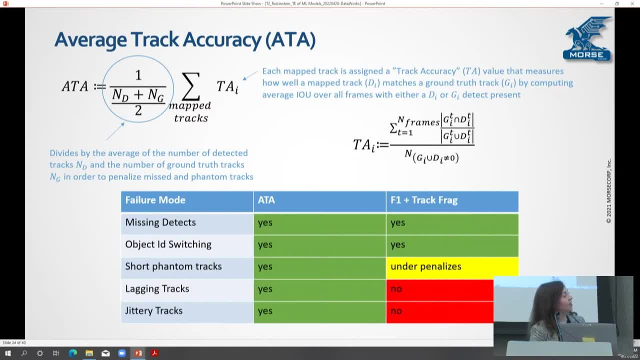 metrics You can see that ATA adds a number of different failure modes that it's looking for and trying to tamp down on. So this again raises the bar, moves the carrot a little bit for the vendors and really gets at that spatial alignment. 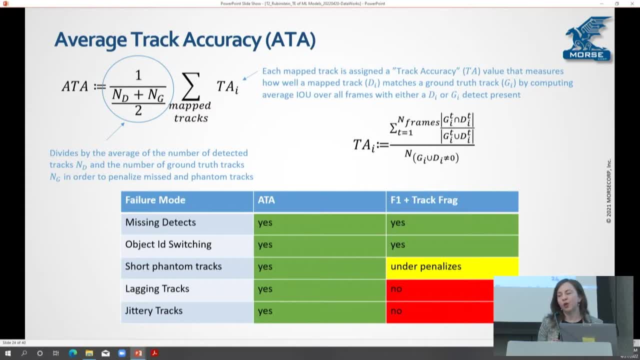 that spatial alignment that ATA is looking for and trying to tamp down on. So this again raises the bar, moves the carrot a little bit for the vendors and really gets at that spatial alignment that that, on its face, might not seem so important. 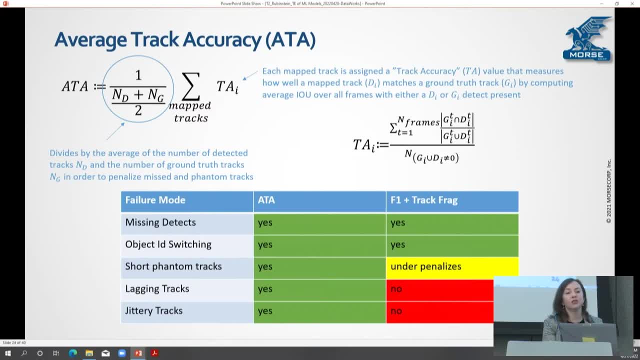 If the detections are close, why isn't that good enough? But if you're actually trying to use the information that AI is giving you, especially in real time on something like a video, those spatial alignment things, can be really important and can really matter to you. 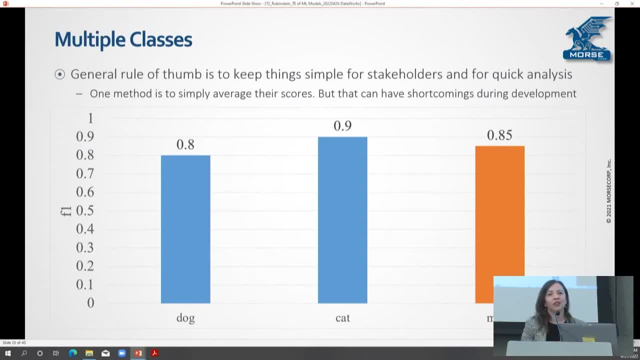 Okay, so let's say you've come up with a good metric for your one class. Now what do you do when you have multiple classes that you're trying to weight and consider the value of? So something simple and easy to do is to just average them all together. 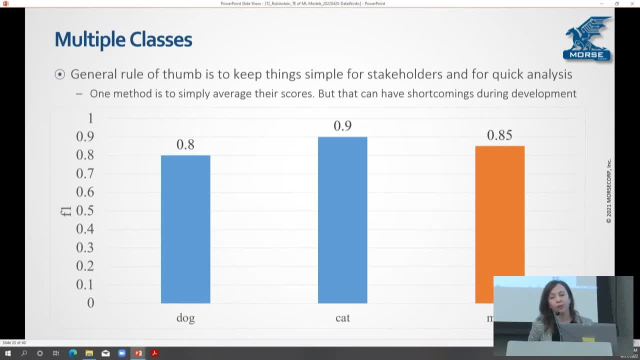 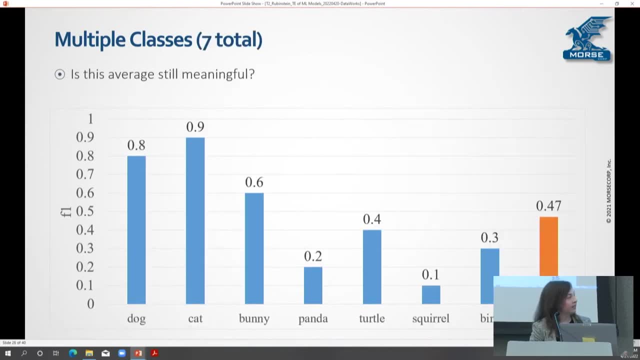 And that can make a lot of sense when you have performance in different classes that are pretty similar and equally weighted. But what happens as you continue to add different classes that have really variable performance? Would an average of the performance across all of these different classes still be meaningful? 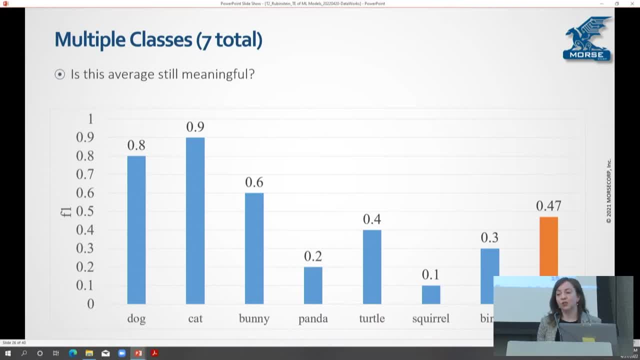 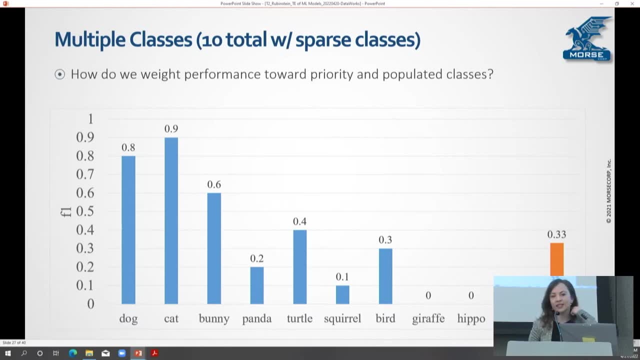 Does that really tell you anything about how you, as an individual user, might wanna use this model? And then, as you continue to add, what if you're adding classes that aren't very populated in data? It's telling you more about the state of your data. 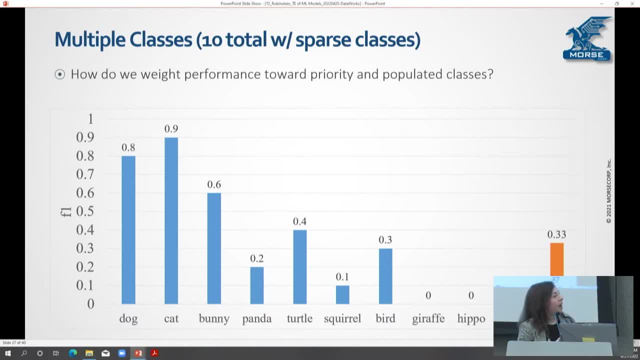 than the performance of your model, necessarily. But again, how do you take all of these different classes into account? And I don't think there's any one size fits all solution here. It will base on what the priorities of your users are and the priorities of your program. 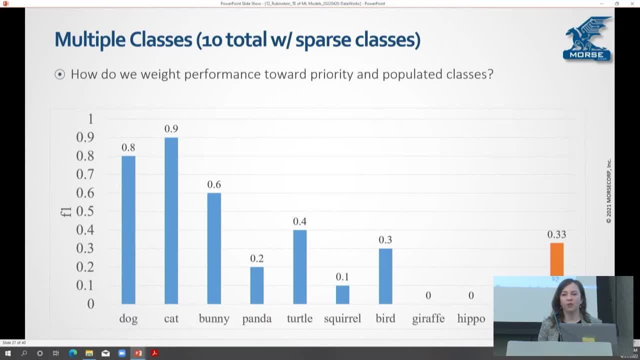 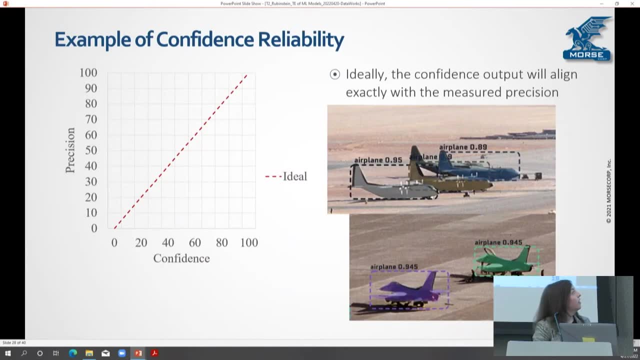 If you're focused more on R&D at that moment than producing something functional for a user, you might make different choices about which of these classes you care about, And then switching gears a little bit to. something else that Colonel Woolley talked about is confidence, reliability. 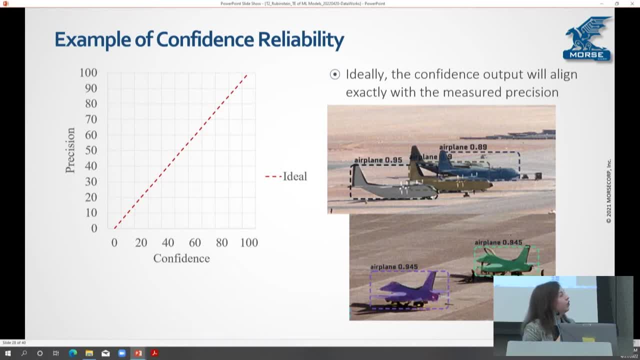 So this is something that can be a very gnarly issue, because it's something that seems like it makes sense to a user but is often really misinterpreted, And that is what the confidence of the individual detections are. A user wants to look at that and say, okay, well, 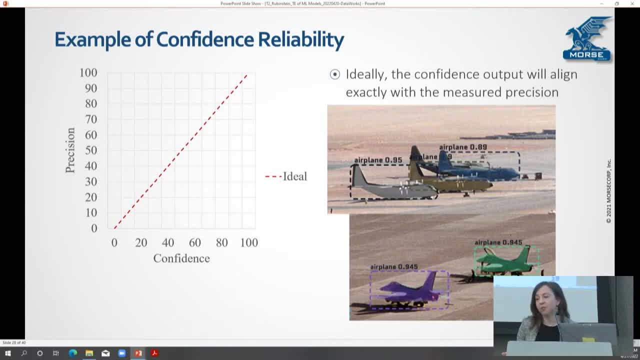 if the AI says, oh well, I'm gonna do this. if the AI says it's 95%, sure, that's an airplane, I believe it, it's an airplane. But you wouldn't necessarily take everything a human told you at face value either, and you shouldn't. 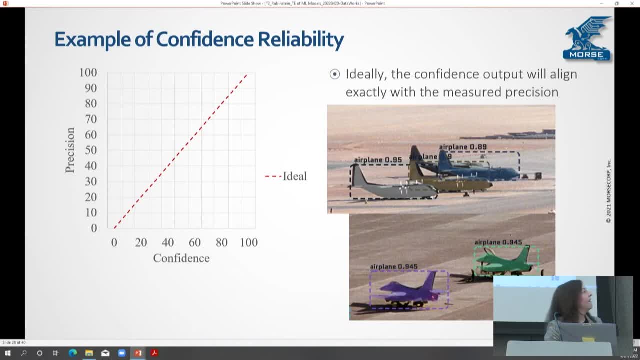 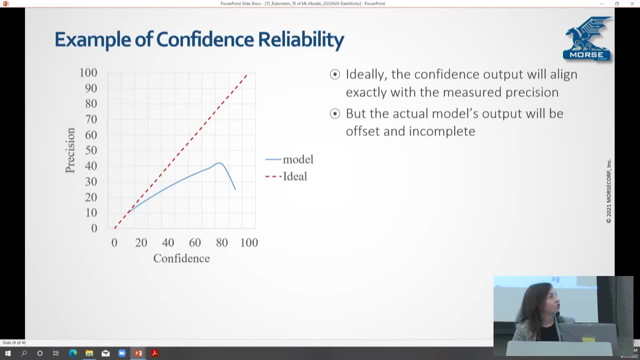 But I think we expect models to be a little bit more self-aware. So ideally the confidence output would exactly align with the measured precision, but actually a model's output often deviates from this And you can measure the error between those curves. 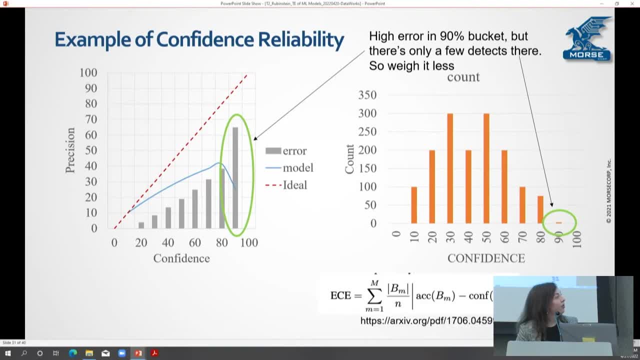 and you can quantify it by how many examples that you have and you can come up with metrics. We have ECE- expected confidence error. that can help you sort of get a sense of how off a model is And if you surface that to a vendor. 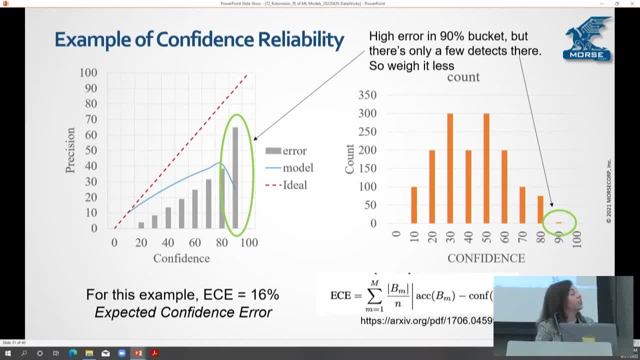 they can try to take that into account and make some adjustments in the confidence values that they output. So hopefully those numbers start to actually reflect what users often interpret them to mean. All right, so now I'm gonna talk about some T&E capabilities. 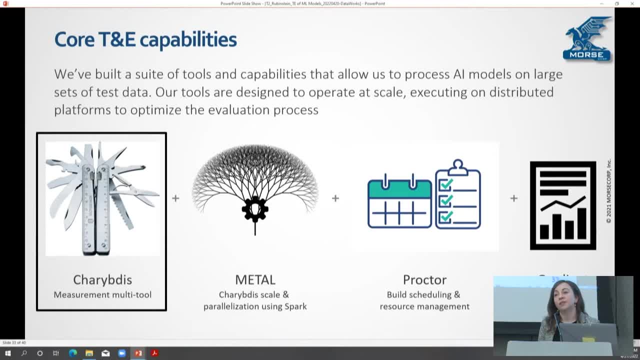 for how you could actually implement those metrics successfully from a T&E as a service perspective or an enterprise-wide T&E perspective. So at Morse we've built a number of different tools to get at different pieces of this. We have Charybdis and that's kind of our Swiss Army knife. 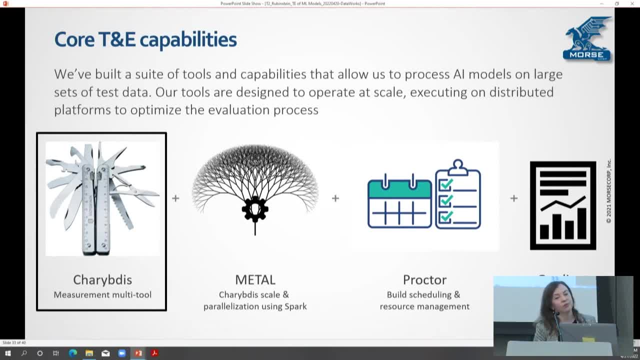 of T&E capabilities. We have Metal that enables Charybdis to run using parallelization so really quickly. We have Proctor that does the scheduling and resource management of the computational resources, And we have Gradient, which turns all of those T&E results into visuals. 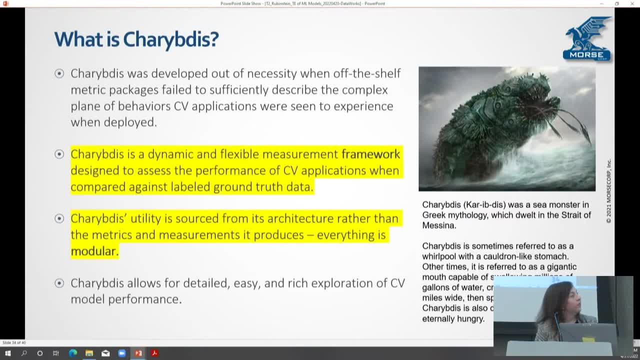 I'm gonna dive into Charybdis a little bit. The reason why that name was chosen is because Charybdis is a sea monster that is eternally hungry, So you can think of our capability as being eternally able to consume models. 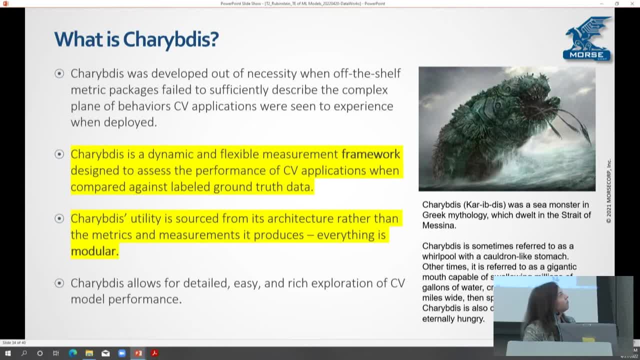 and to spit back out these T&E results, And so it was developed out of a need, because no off-the-shelf package would really deliver the full suite of capabilities. So that's why it's called Charybdis. And then we have the T&E analysis that we were looking for. 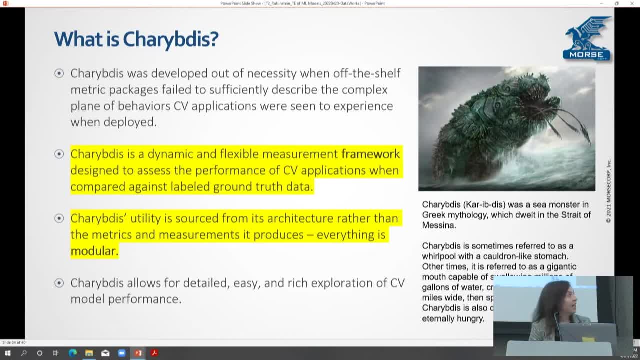 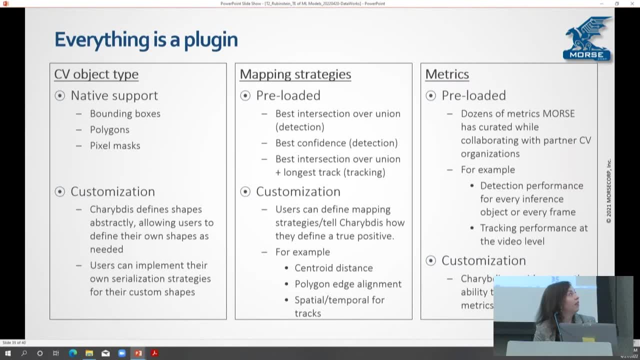 And ultimately it's a framework. It's a flexible and dynamic framework for doing T&E analysis of CV applications, And so it's modular. Everything is plug and play into the system, So I'll highlight that here. So, in terms of the CV object types that it can ingest, 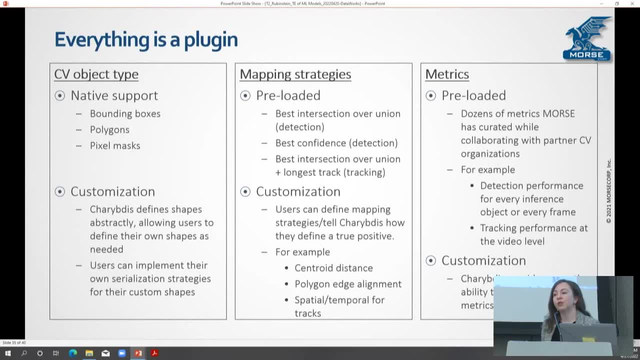 it can handle bounding boxes, polygons, pixel masks, And that's important. It's important to be able to be flexible across those. It can handle bounding boxes, but half of your labeled data is polygons. How do you mesh them together? Well, Charybdis can handle all of these different types. 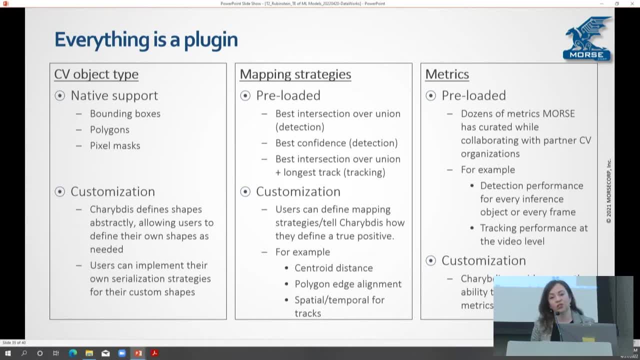 of object types And it even allows customization so you can program in your own shapefiles. It also has different mapping strategies that might also change depending on your use case. How do you choose if you have multiple boxes overlaying a ground truth? How do you choose which one you map together? 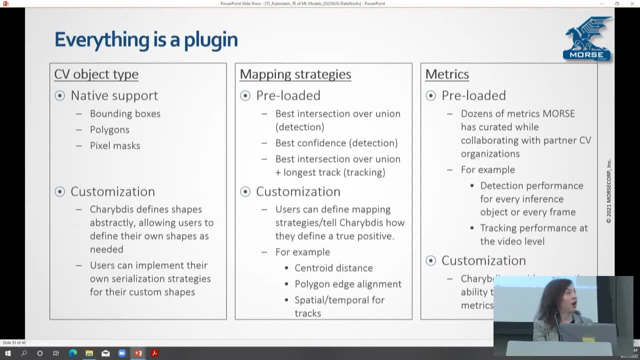 Is it the best intersection over union? Is it the best confidence? The user is allowed to choose those kinds of things, And if anything that's natively available isn't what you want, you can program your own choice. And then, in terms of the metrics themselves, 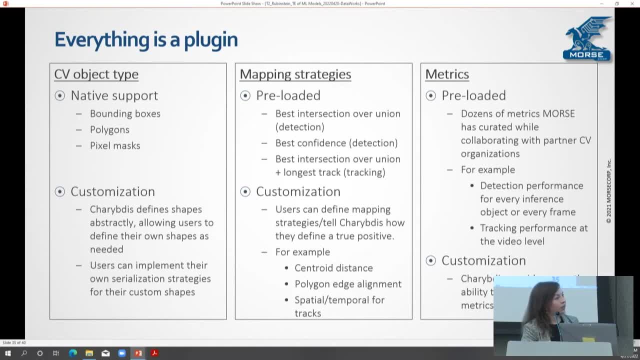 a number are preloaded, Some very common ones that are used across many programs. But if you need to customize your own, you can, And you can also figure out how you want to apply those metrics. Do you want to apply it over every object? 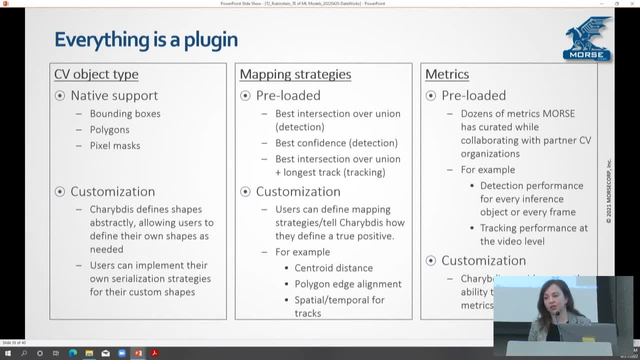 Yeah, Or every frame, Or across an entire sequence. Different choices make sense for different types of models, And you're allowed to facilitate those with Curbdisc, All right. so I just wanted to take a few minutes and talk about some best practices that. 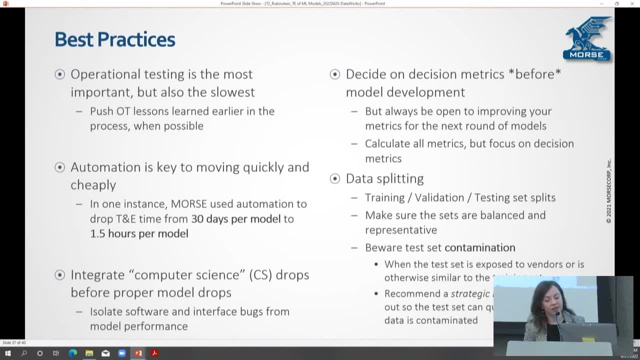 have been learned over time here. So, as Colonel Willie mentioned also, operational testing is the most important, but it's the slowest, So it's easy to push that off until the end, but that's not the best way of doing it. 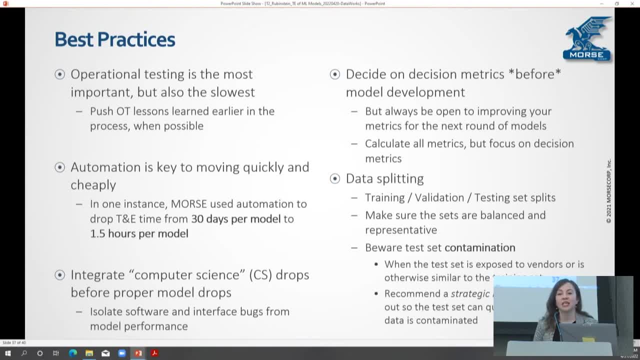 It's really better to do it as early in the process as you can, even if you have something that's not fully functional yet, just to start getting those lessons learned, so you don't get too far down the rabbit hole that's taking you in the wrong direction of something that's 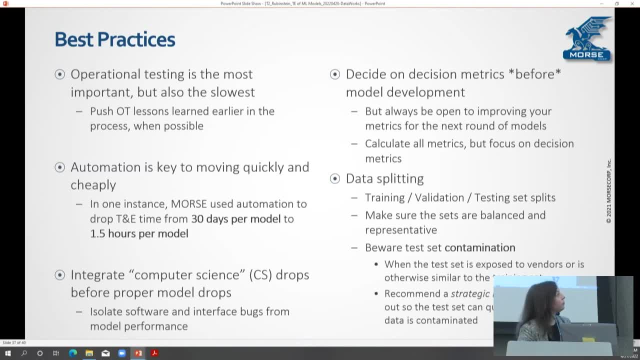 not going to be important to users, So try to do it as early as possible. Automation is very key to moving quickly and cheaply And a lot of the lessons learned I highlighted here already. A lot of the frameworks that we've built are built specifically. 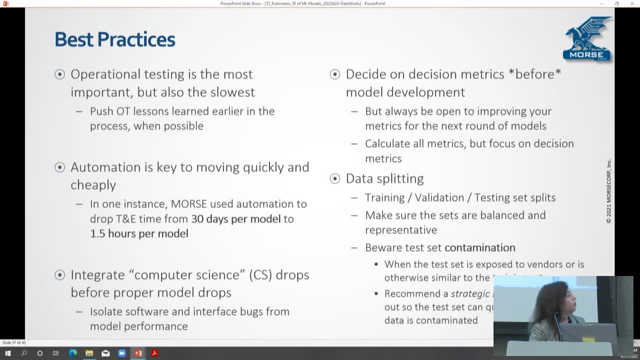 to facilitate this. this speed, Because we want things to be sitting with humans as little as possible, And passing that information back and forth quickly is very key to getting rapid innovation and success. It can also be really helpful to integrate computer science drops before proper model drops. 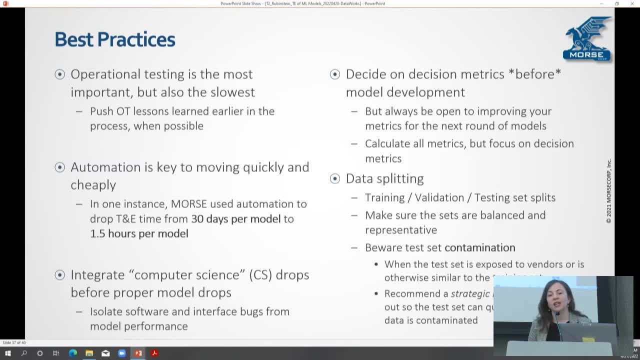 And so what's meant by that is, if you have a lot of system integration, it's good to do a drop early in your sprint cycle that doesn't have the fine-tuned weights that you'll get at the end of your sprint, but has enough. 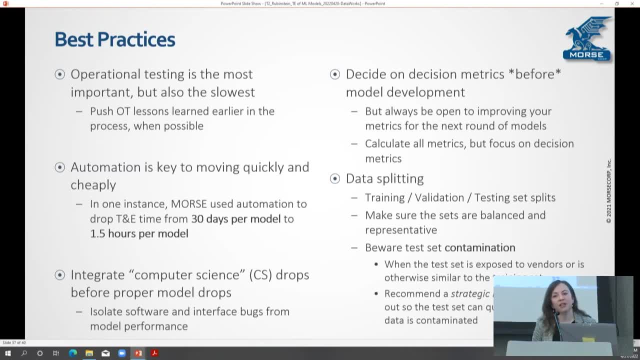 of the infrastructure there so that if you need to get any certifications to field any certain IA processes that you're trying to run, you can do those early and up front And then substitute in the final model weights at the end. But that can help identify a bunch of software and interface bugs early. 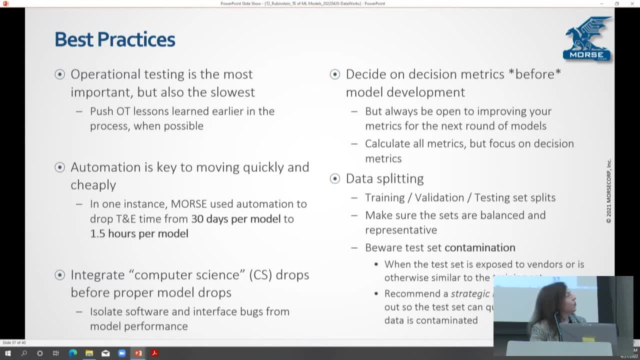 which is really important, And so another one is: you want to decide on your decision metrics before you start model development, but you have to be open to like improving and evolving over time. As I mentioned a number of the different metrics that we've used, we could not have possibly. 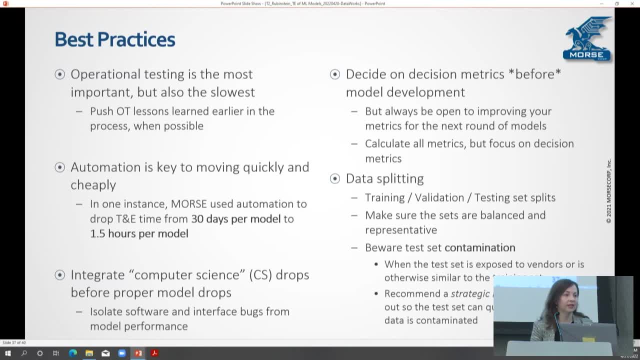 known why they would be important or necessary at the beginning. So it's something that you should always be looking at, I think, each sprint, taking a critical look at what you've learned, how far the models have come, what users are asking for. 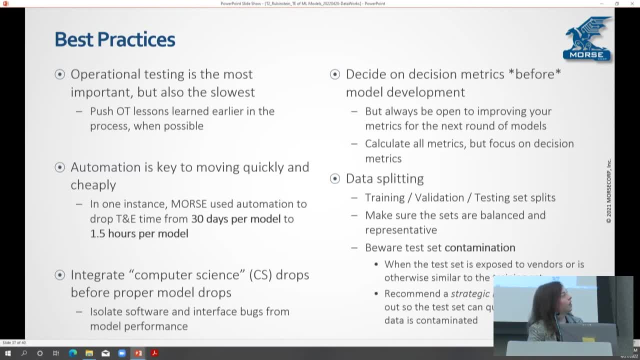 and then making a choice based on that. And then it's important to calculate all metrics. Even if you do just calculate those decision metrics that are very, very rolled up, it is very important to unroll them and to look at what the performance on the different components is. 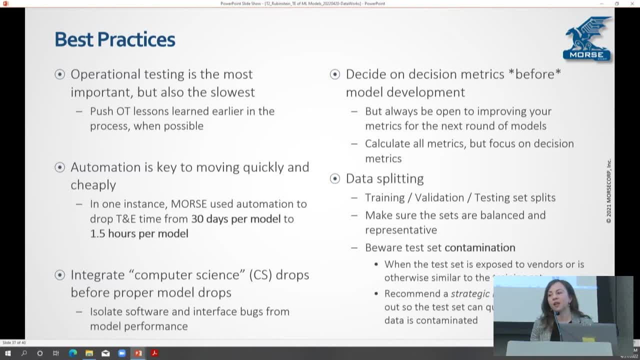 because you don't want to blur things and lose that transparency about how models are actually performing. A lot of that nuance can get erased if you're not careful, And then data splitting is important. You want to have test, train and validation set splits. 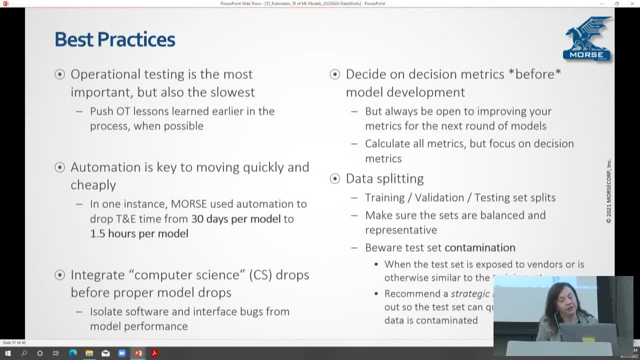 Make sure they're balanced and representative And be very, very careful about test set contamination, because you know, once it's lost you can't get it back And it can be a good idea to have a strategic reserve that you hold just. 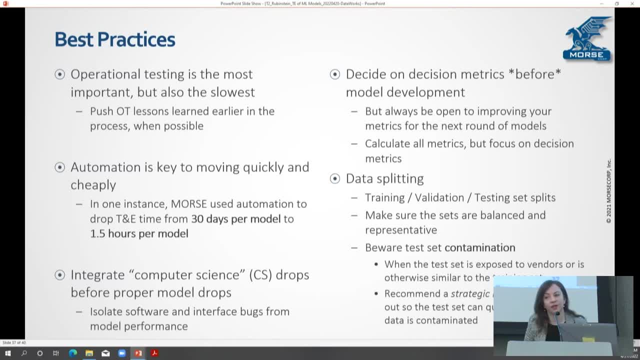 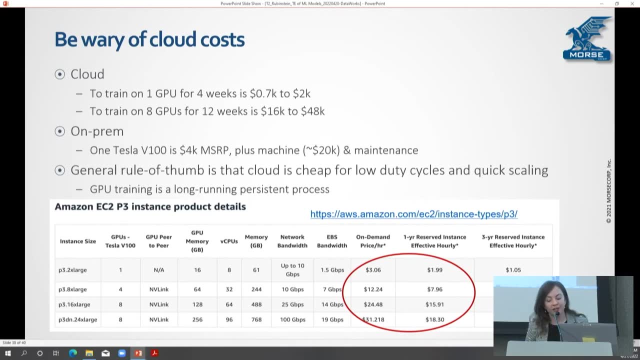 in case mistakes like this happen, because unfortunately it does more than we would like. And then, just another note is to be wary of cloud costs. There's a real conversation to be had about the tradeoffs between on-prem compute resources versus the cloud. 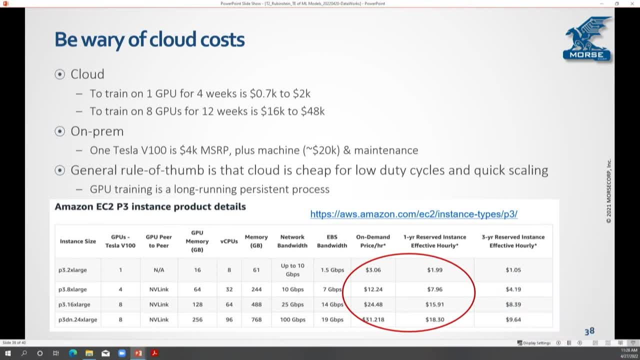 Cloud costs can scale quickly, and so you need to be cognizant of them, and you also need to think about how you want to manage cloud resources. Do you give it to the vendors themselves so they can have that rapid scalability you know, at will? 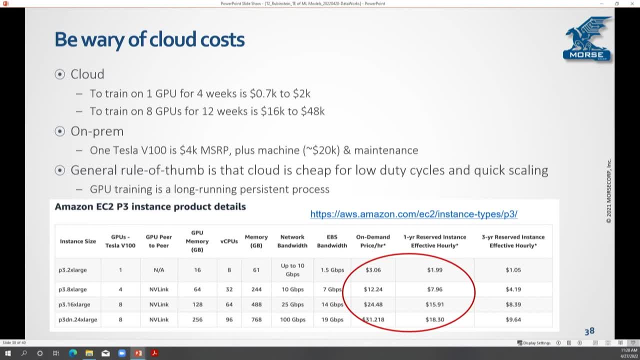 Or, you know, do you trust them with the budget? Do you want to hold that closer to yourself? You know, again, those are conversations that just need to be thought of, the most effective way to do these things. All right, and this is just some link to available libraries. 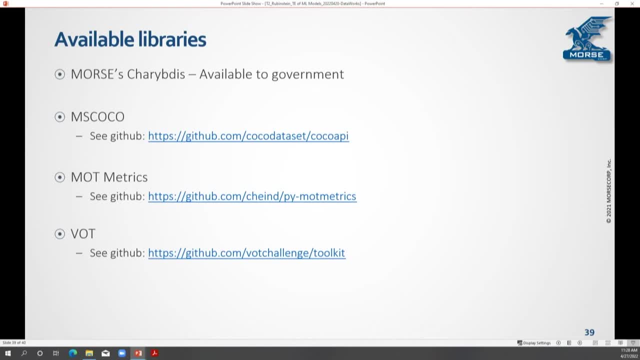 for computer vision metrics. So with that I will stop, And I think I probably do have time for any questions. Thank you, Anna, And while Caitlin checks to see if there are questions in the room, I love the description of Charybdis. 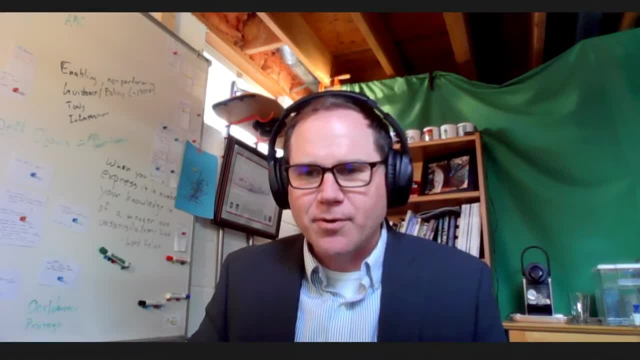 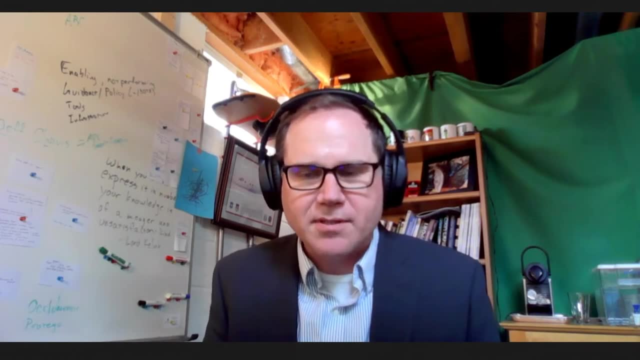 as being eternally hungry. I don't think I'd heard it actually defined in those terms before. I see that Charybdis is available to the government. Do you know if Maven has a plan for how to release or distribute those to interested parties? 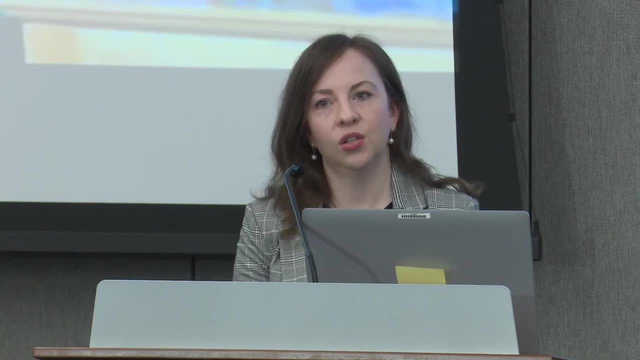 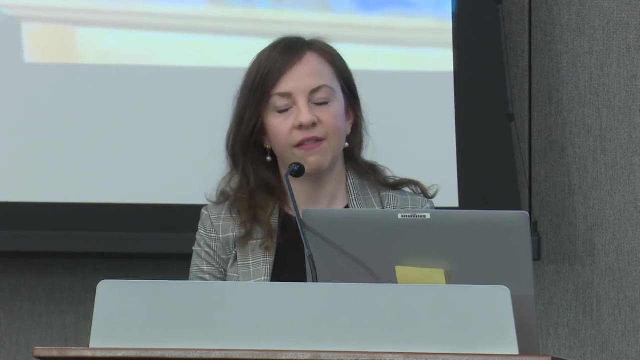 I don't. I don't know that it would necessarily go through Maven specifically Or through Morse, but if anyone you know reached out and was interested, we could have that conversation and set that up If we were interested in making them available. 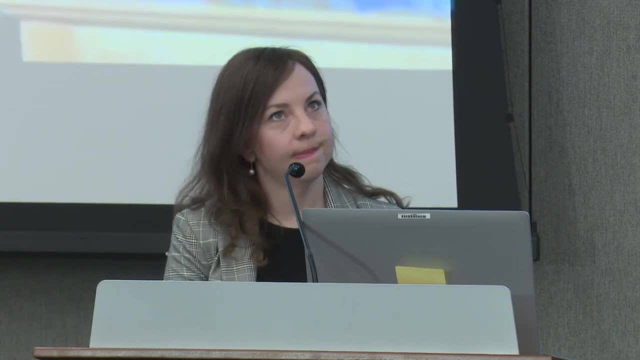 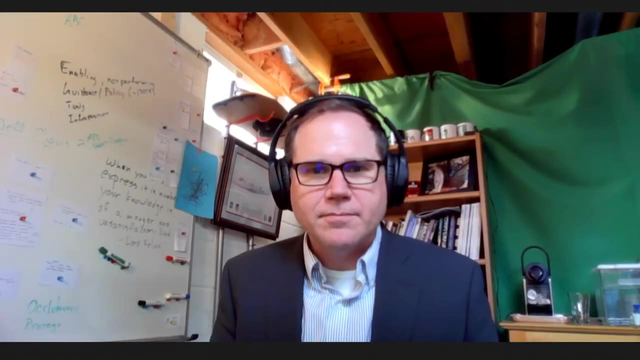 through Iron Bank or one of the other government distribution methods. is that something that you think they might be interested in, Or do you want to follow up with me and see if that's something we could check into? Yeah, I know I've heard Iron Bank mentioned before. 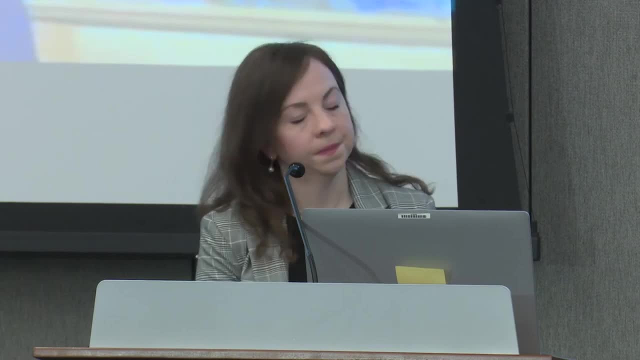 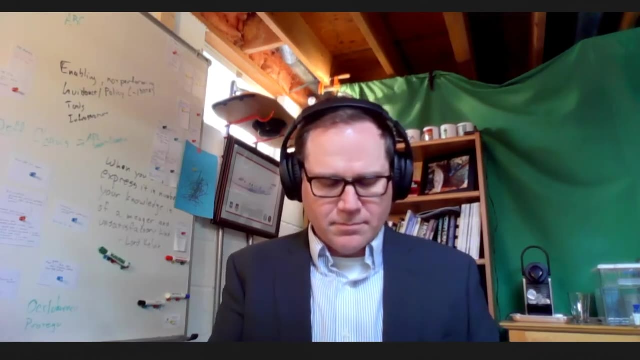 so we can check in on that and I'll see. Thank you, Caitlin. do you have any questions? I don't see any questions from the room. Howdy Sam McGregor with AfoTech. So you mentioned using the computer science drops. 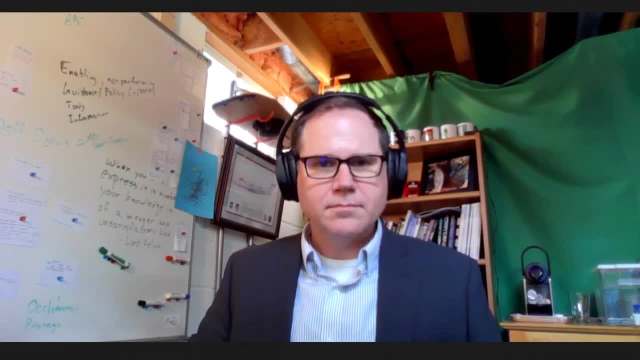 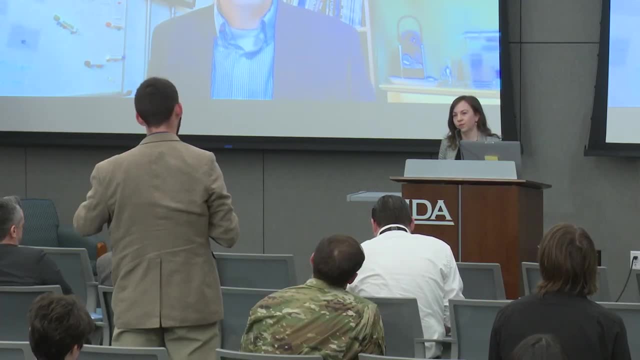 to work out bugs and all that sort of thing beforehand. The next step up I'm seeing is that: what if you're getting systems interacting where there's no bugs in the systems, but the interaction between those systems is creating bad inputs? How are you handling that? 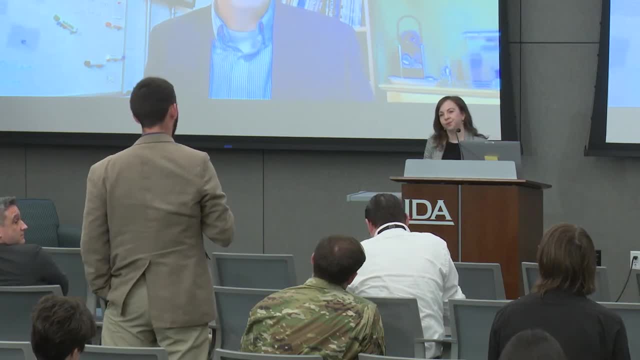 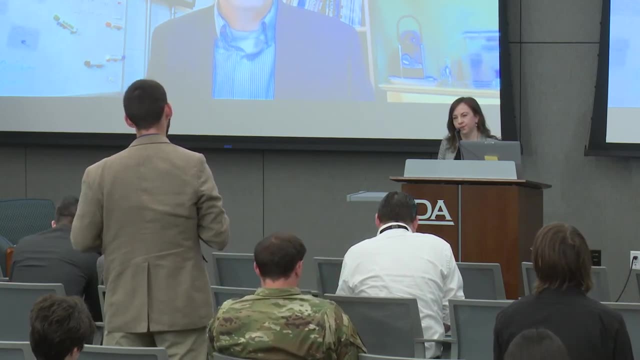 Can you give an example of what you're thinking about? Sure, So one of the examples I was reading about was an ATC system- air traffic control- for it was designed for the United States, However, it was applied in Britain. 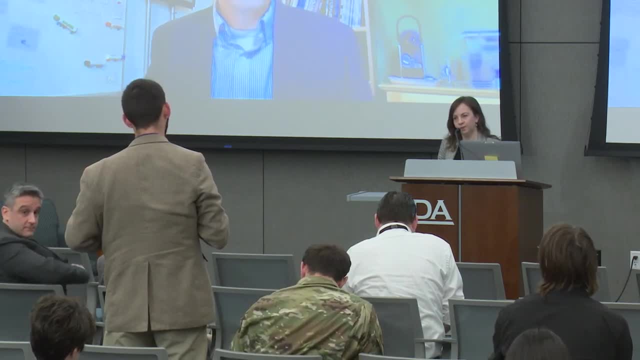 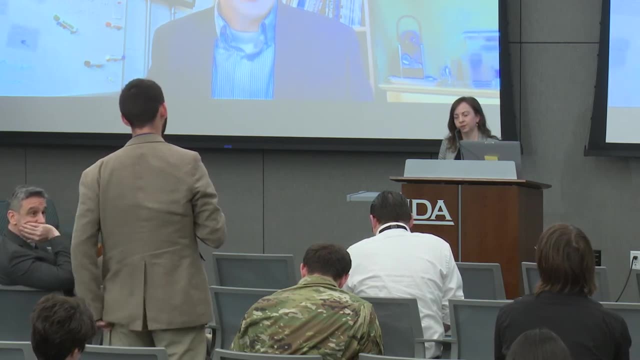 The problem being with the latitude-longitude system, with there being zero right there. the system could not handle that, So it ended up putting effectively the coordinates for one town over another. Huge issue, right. How are you countering that in your systems? 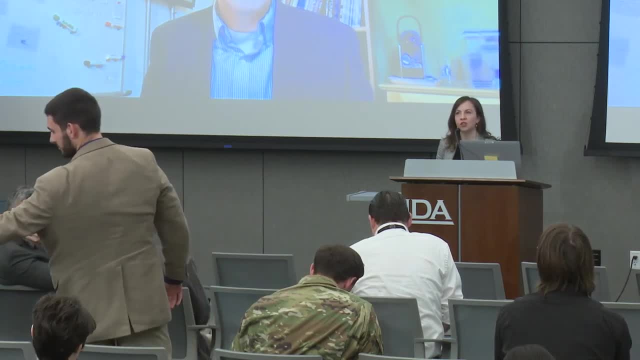 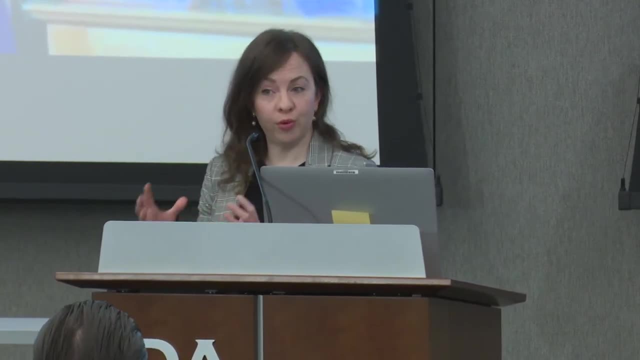 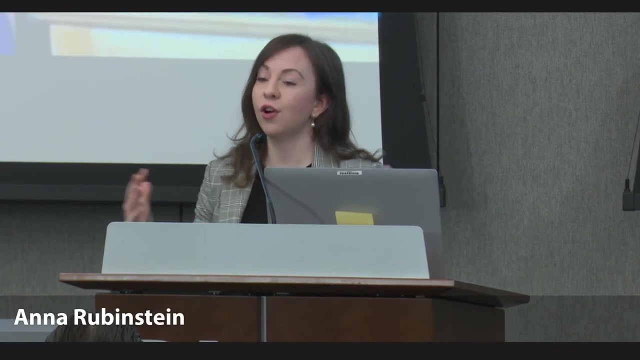 Right. So we haven't encountered that too much just because the models that we've developed plug into, you know, UIs and systems that are also developed for our programs specifically. But absolutely I would expect issues like that to happen if we were integrating even farther afield than that. 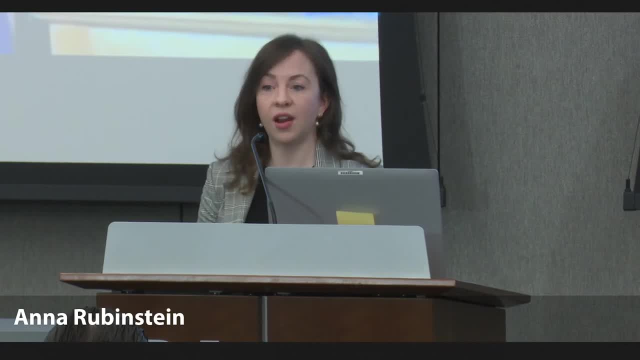 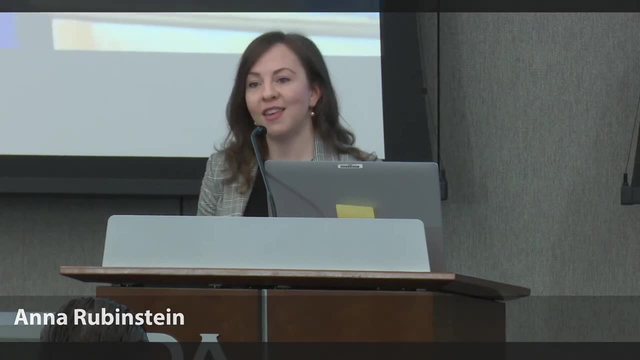 into third-party systems, other programs of record. So issues like that are going to happen when you try to do these integrations, And I think it would just be, you know, trial and error. I mean, I think both sides would need to communicate as much. 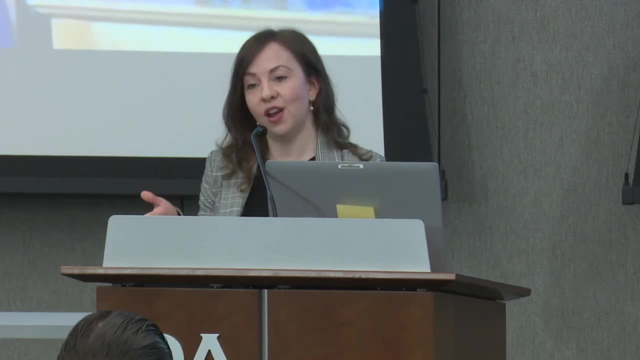 as possible about. you know what the outputs of one system are and the inputs of another. But there are going to be missteps like that And I think you just have to- you know, to be on the lookout for them and make sure. 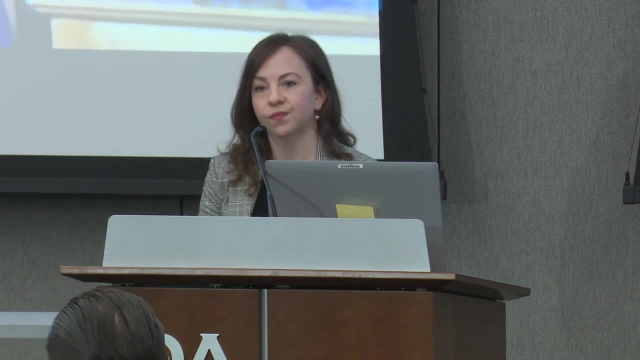 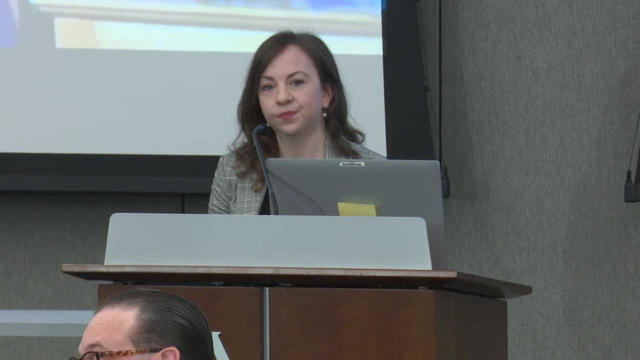 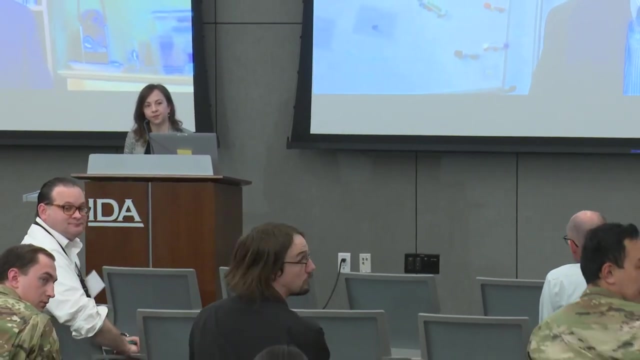 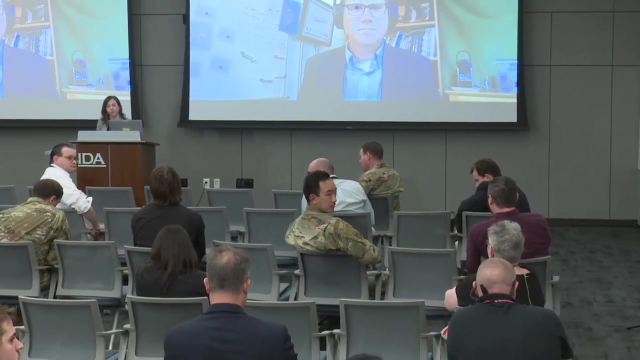 that all your outputs make sense. Hi, Breonna Anderson, with IDA, I was wondering if you could speak to how Charybdis handles learning over time specifically. So these models, These models aren't static right, They're learning. 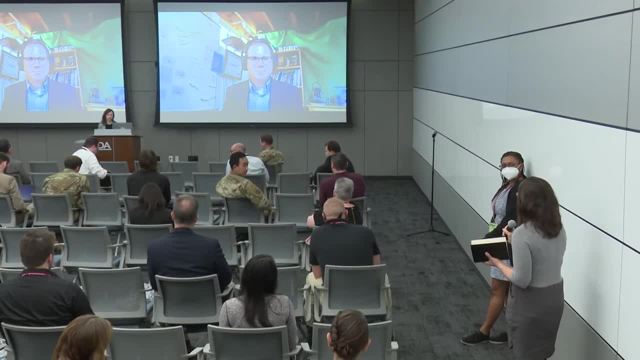 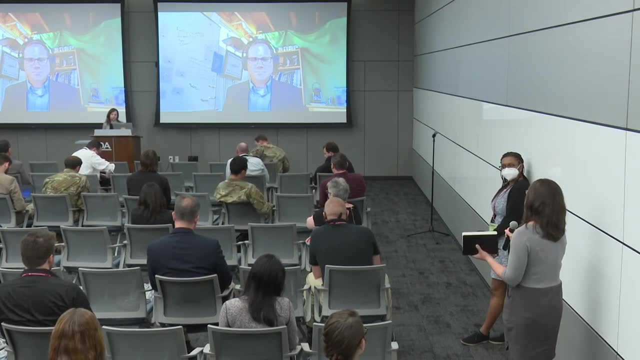 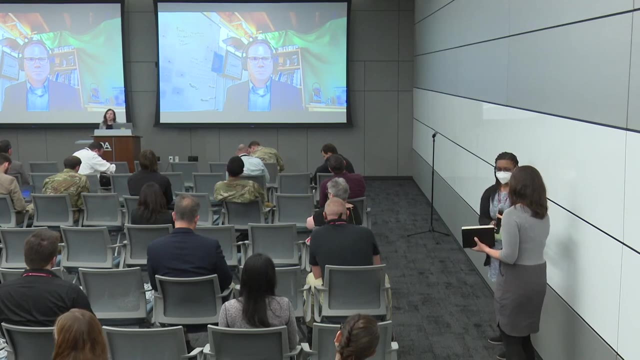 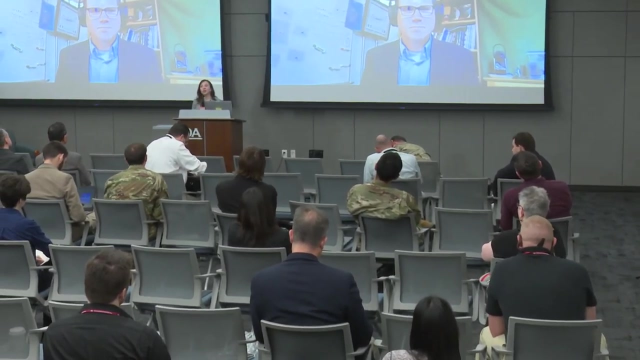 And so I would imagine that the metrics are changing as well. And so how, within your data sets, are you handling the change in the metrics and the learning over time with these programs? Right, So to be clear, the models, the way they're deployed. 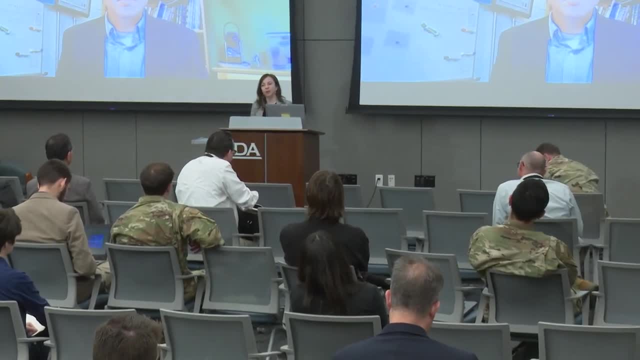 they're deployed frozen. So whatever weights have been set up, you know they're frozen, They've been tuned up to that point, are frozen And that is how it is deployed into the field. So once the models are deployed into the field, they're not changing anymore, But each sprint, each 90 days, the vendors are taking all of the additional data that has been provided, you know, by the program and tuning their models to make them even better. So there is continuous improvement. 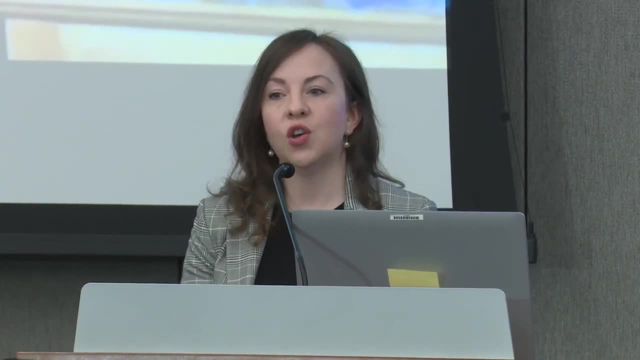 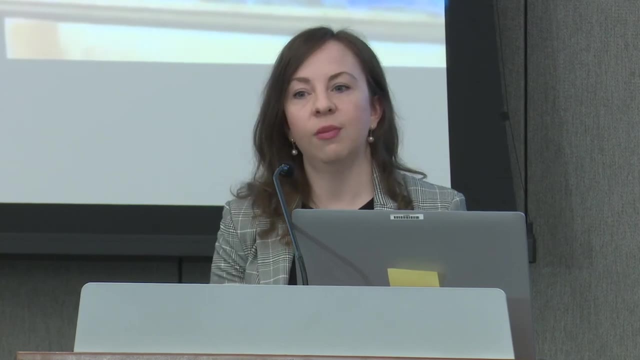 but just with different model iterations. And so each sprint we do another round of T&E where we look at the model performance, you know, over any additional capabilities that have been developed. So if there are new object classes that it can handle, now you know. 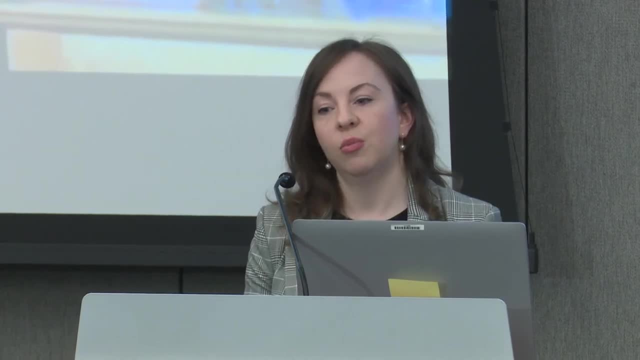 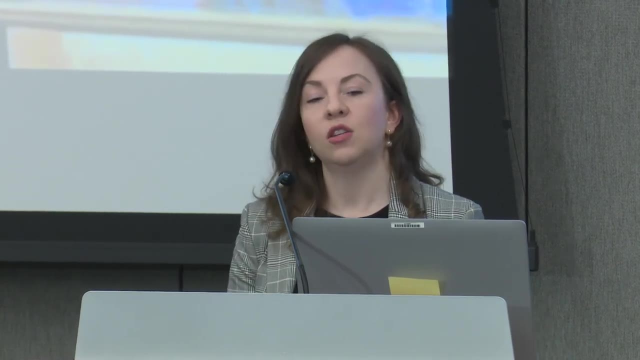 we look at that, We compare it to performance on the previous sprint's model, on that updated data, so that we have a really accurate baseline. You know we use that to set goals. Sometimes we even benchmark against, you know, human level performance. 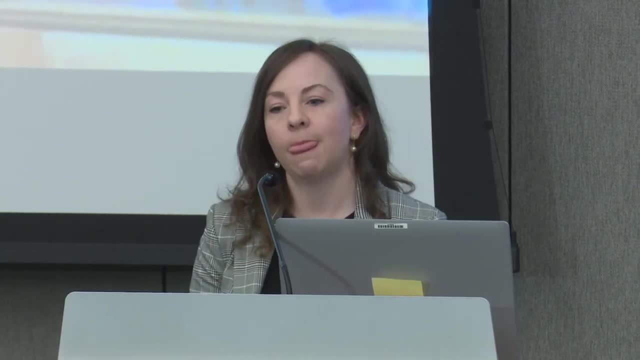 what we would expect on some of the different object classes, And that increases the performance. So we look at the model performance over any additional capabilities that have been provided, So that increase in performance is often what we do to say like okay. 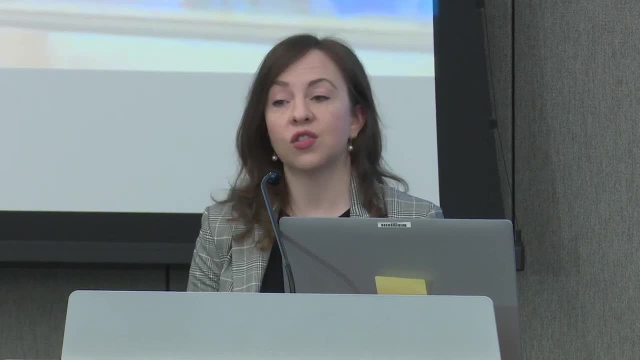 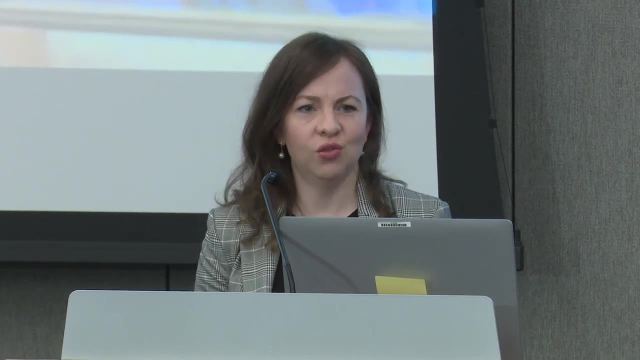 is it time to add additional metrics? When vendors got really good at, you know, the F beta and track frag, it's like, okay, well, how do we like? we know the models visually aren't perfect yet Like: what more do we need to be adding? 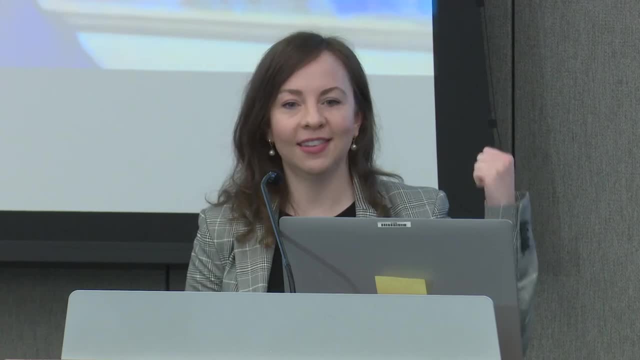 What are we missing? What are we not, you know, putting into math and asking them to do that is still important to users, And so that's when we introduce ATA, and that's new, But that is, you know, designed to do that.